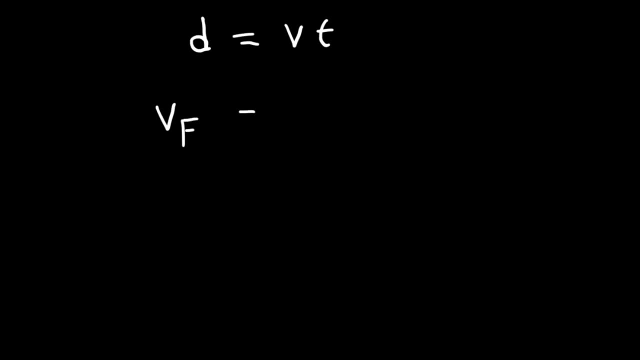 need to know. The final speed is equal to the initial speed plus the product of the acceleration and the time. There's also this equation: The square of the final speed is equal to the square of the initial speed plus two times the product of the acceleration and the displacement. Displacement- 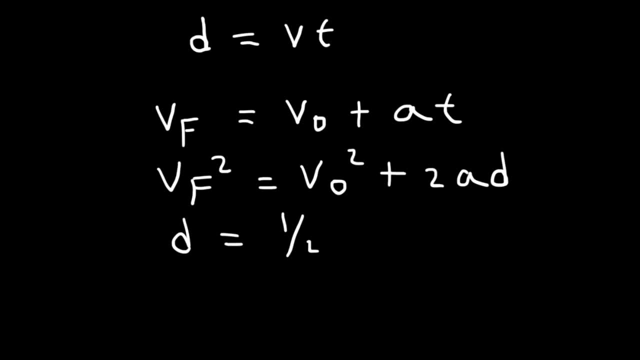 is equal to the average speed, which the average speed is basically the sum of the initial speed and the final speed divided by two, multiplied by the time. As you can see, the third equation that I listed here looks like the first equation for a constant speed. 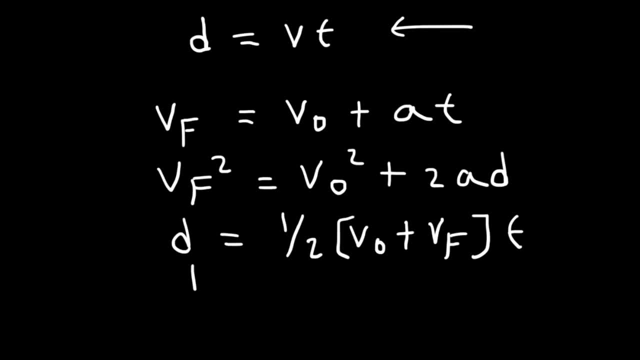 Okay, I did not want to do that, So I can rewrite this equation like this: V average times t, where v average is initial plus final divided by two. Now there's another equation that you need to know: d is equal to v, initial t plus one half a t squared. So make sure you know that equation too. 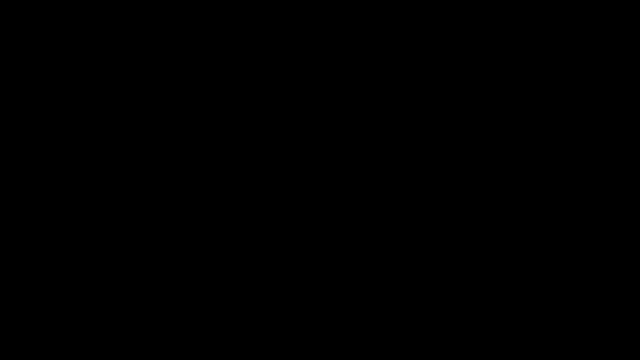 So what exactly is d? You can use d as displacement or distance. Distance and displacement are the same if an object moves in one direction and doesn't change direction. If it changes direction, then displacement and distance is not the same, But technically d is displacement. 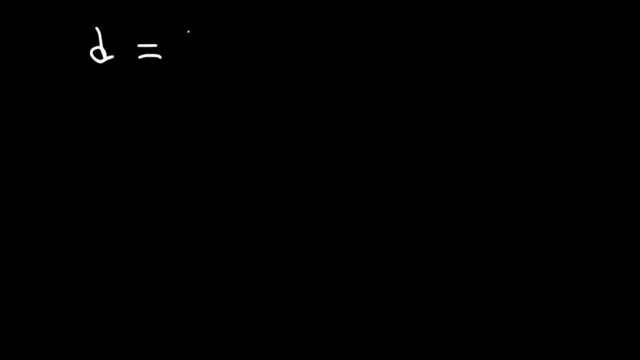 Displacement is basically the difference between the final position minus the initial position. Now you can use displacement in the x direction or you can use it in the y direction, So just keep that in mind. Now there's three types of shapes for projectile motions that you need to be familiar with. Let's say, if we have an object, 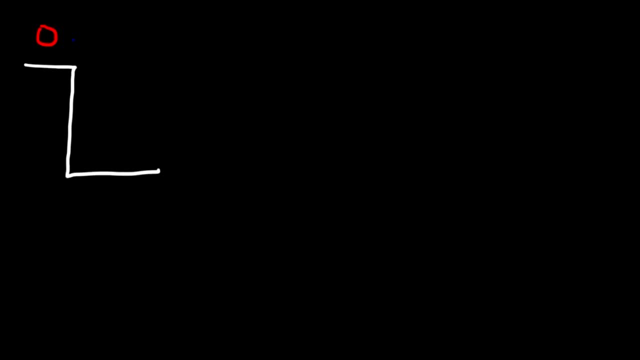 and it comes off a cliff horizontally and then eventually hits the ground. That's the first type of trajectory you're going to be dealing with. So what equations do we need for this situation? The first equation that's going to help you is this: h is equal to one half. 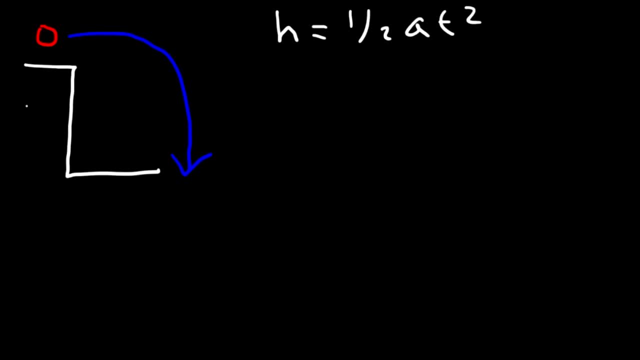 a- t squared, where h represents the height of the cliff and t is the time it takes to hit the ground. This equation comes from this equation: d is equal to v, initial t plus one half at squared. Now, when you're using these equations, you need to ask yourself: 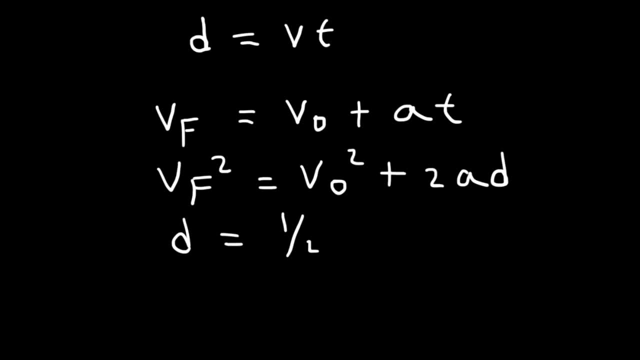 is equal to the average speed, which the average speed is basically the sum of the initial speed and the final speed divided by two, multiplied by the time. As you can see, the third equation that I listed here looks like the first equation for a constant speed. 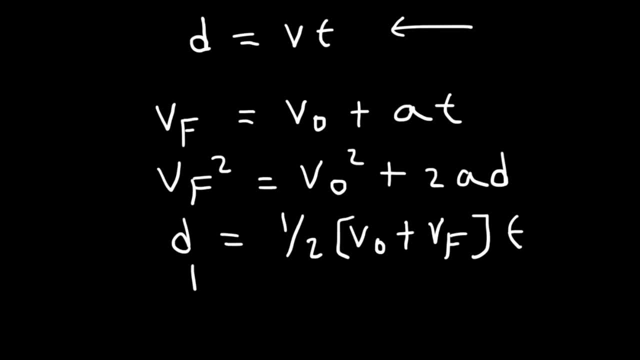 Okay, I did not want to do that, So I can rewrite this equation like this: V average times t, where V average is initial plus final divided by two. Now there's another equation that you need to know. to just know, D is equal to uh, V initial t plus one half at squared. So make sure you know. 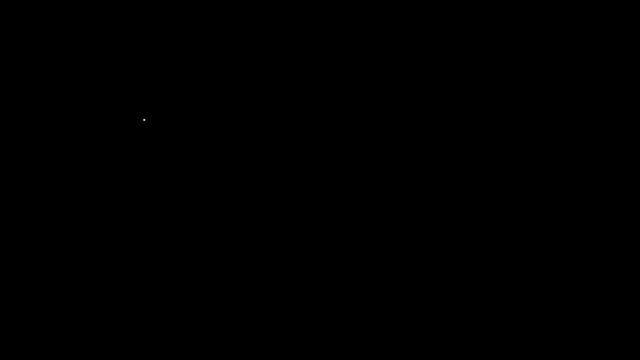 that equation too. So what exactly is D? You can use d as displacement or distance. Distance and displacement the same if an object moves in one direction and doesn't change direction. if it changes direction, then displacement and distance is not the same. but technically d is displacement. 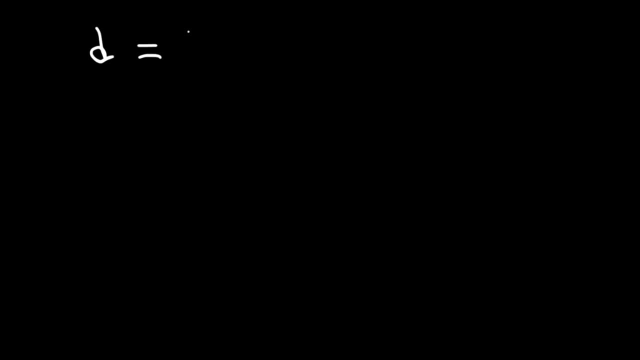 displacement is basically the difference between the final position minus the initial position. now you can use displacement in the x direction or you can use it in the y direction, so just keep that in mind. now there's three types of shapes for projectile motions that you need to be familiar with. 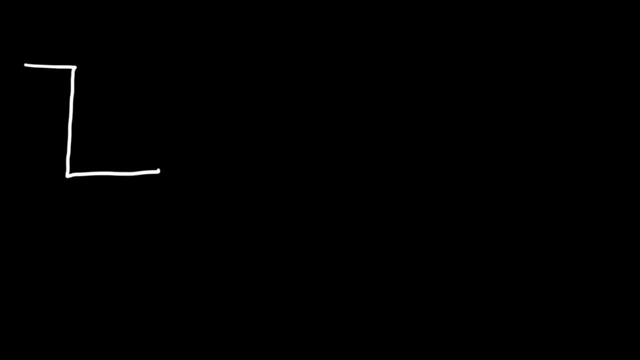 let's say, if we have an object and it comes off a cliff horizontally and then eventually hits the ground, that's the first type of trajectory you're going to be dealing with. so what equations do we need for this situation? the first equation that's going to help you is this: h is equal to one half. 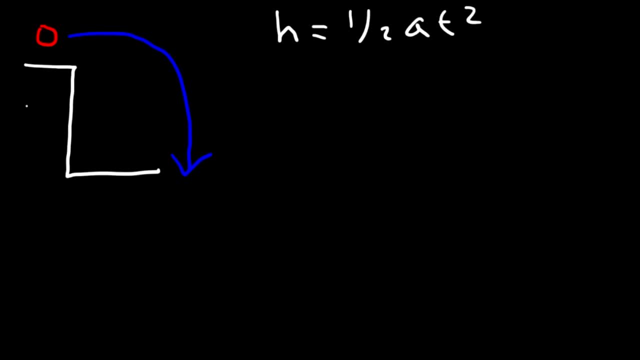 a t squared, where h represents the height of the cliff and t is the time it takes to hit the ground. this equation comes from this equation: d is equal to v, initial t plus one half a t squared. now, when you're using these equations, you need to ask yourself: 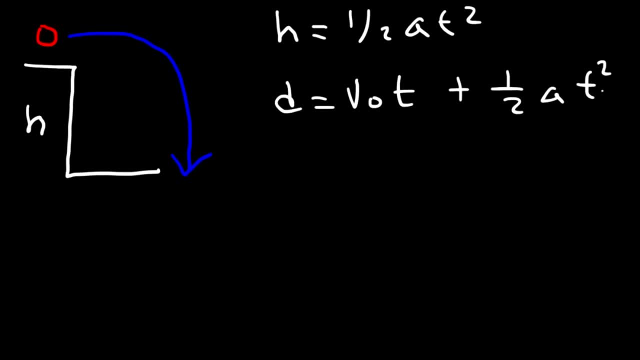 am i dealing with the x direction or the y direction? you got to separate x and y for projectile motion problems. we're going to apply this equation along the y direction. so this is really: d? y is equal to v? y initial times t plus one half a y times t. squared d? y, the displacement in the y. 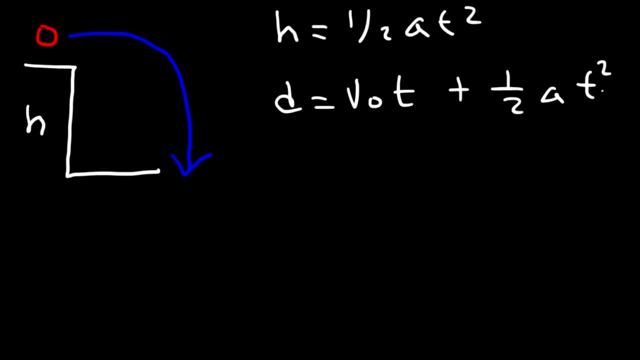 am I dealing with the x direction or the y direction? You got to separate x and y for projectile motion problems. We're going to apply this equation along the y direction. So this is really: dy is equal to vy initial times T plus one-half Ay times T. squared Dy, the displacement in the y. 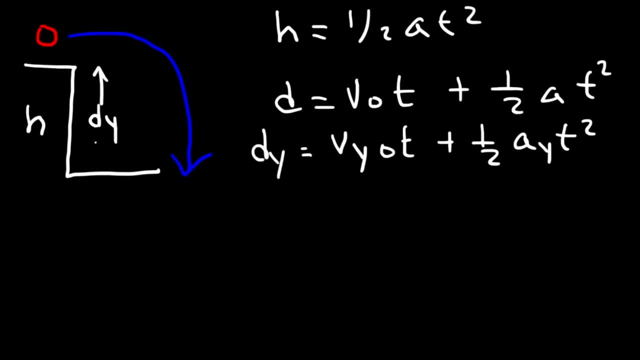 direction is basically the height, So that's H. Vy at the top is always zero, because the object is moving horizontally. The initial speed of the ball is Vx, not Vy, And so we get this equation. So H is equal to one-half At. 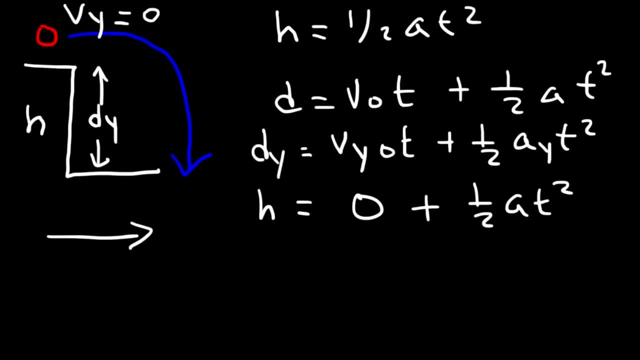 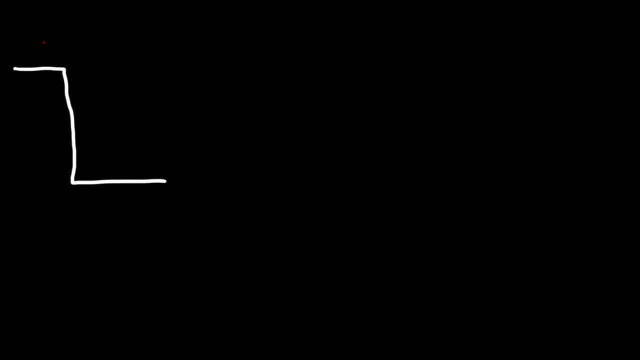 squared. Let me just redraw this picture, So make sure you know the first equation that we just mentioned. Now, in addition to knowing this equation, if you know the time you can find the height of the cliff. There's also another one: We 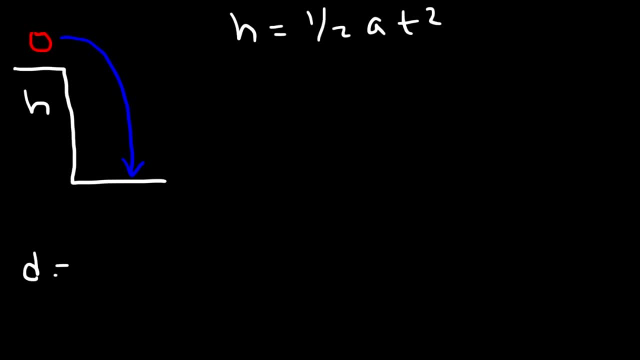 know that d is equal to vt. This is the range of the graph, the distance between where the ball lands and the base of the cliff. Now, if we apply this equation in the x direction, the displacement in the x direction is the range, So we can say that the range is equal. 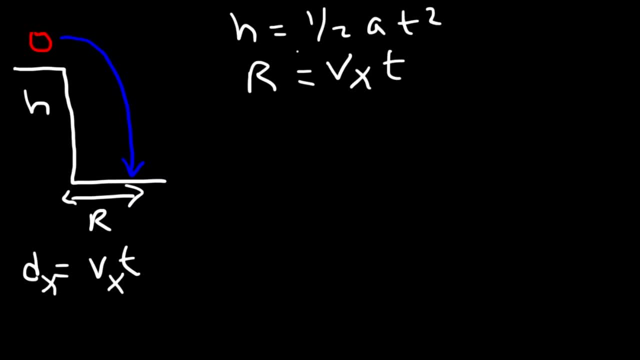 to vxt, And for this type of trajectory, vx is the initial speed of the ball. So that's how you can calculate the range. If you have the range, you can find the time and then, using the time, you can find the height. So these are the two main equations that you'll 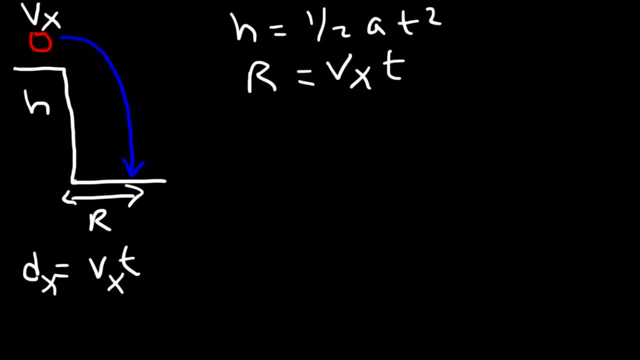 need for this particular trajectory. Now there's some other equations. Sometimes you've got to find the speed of the ball just before it hits the ground. Whatever vx was at the beginning, vx would be the same For projectile motion problems. vx does not change The acceleration in the x direction. 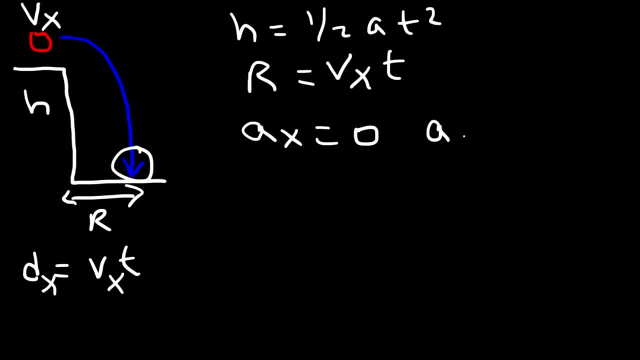 is zero, so vx is constant. The acceleration in the y direction, that's the gravitational acceleration, it's negative 9.8.. And so vy changes To calculate vy. we can use this equation v final equals v initial plus at, But we're going to use it in the y. 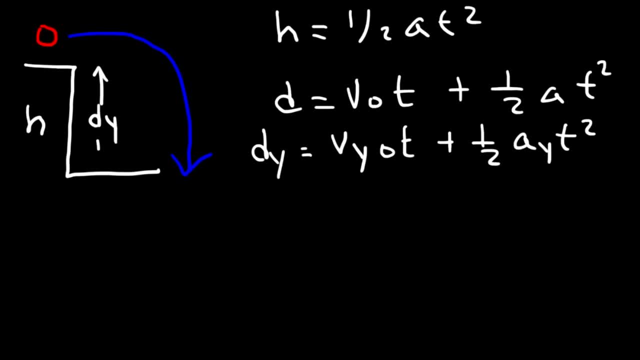 direction is basically the height, so that's h v y at the top is always zero, because the object is moving horizontally. the initial speed of the ball is v x, not v y, and so we get this equation. so h is equal to one half a t squared. 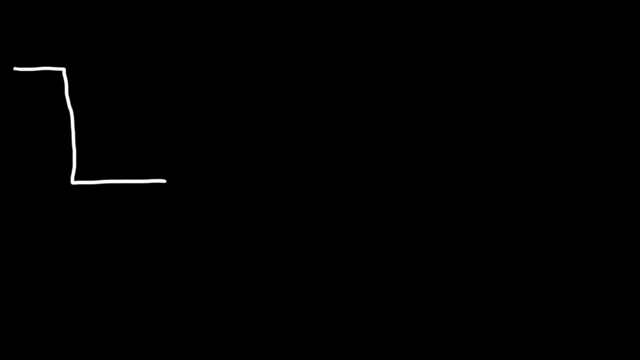 so let me just redraw this picture so make sure you know the first equation that we just made. so this equation is going to be equal to the height of the cliff. now, in addition to knowing this equation, which, if you know the time, you could find the height of the cliff, there's also another one: we know that d is equal to vt. 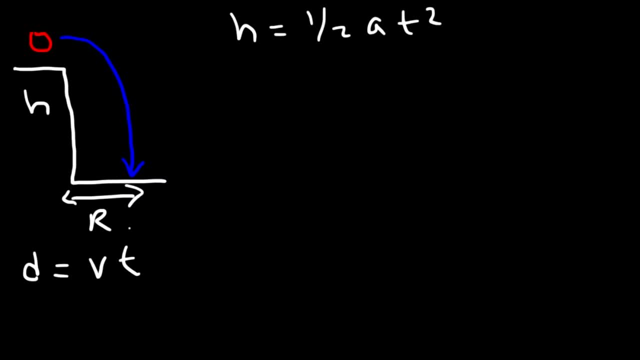 this is the range of the graph: the distance between where the ball lands and base of the cliff. now, if we apply this equation in the x direction, the displacement in the x direction is the range. So we can say that the range is equal to vxt. 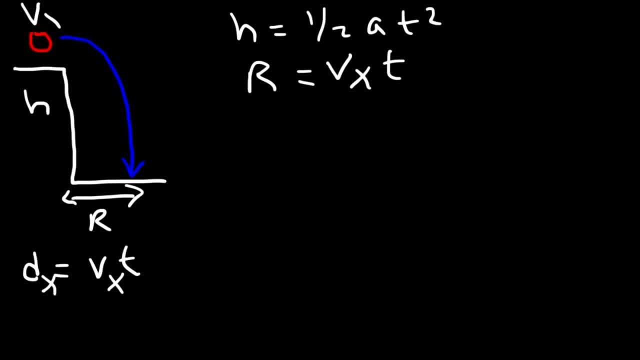 And for this type of trajectory, vx is the initial speed of the ball. So that's how you can calculate the range. If you have the range, you can find the time and then, using the time, you can find the height. So these are the two main equations that you'll need for this particular trajectory. 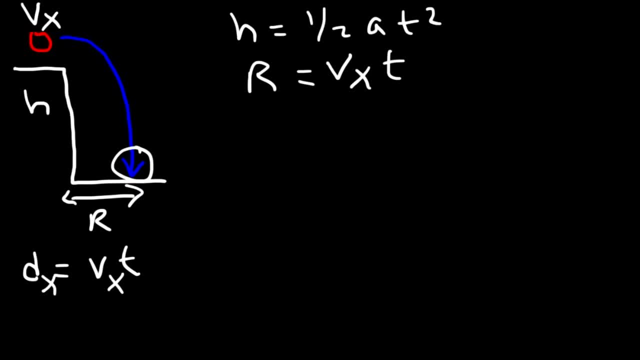 Now there are some other equations. Sometimes you've got to find the speed of the ball just before it hits the ground. Whatever vx was at the beginning, vx will be the same. For projectile motion problems, vx does not change. The acceleration in the x direction is 0, so vx is constant. 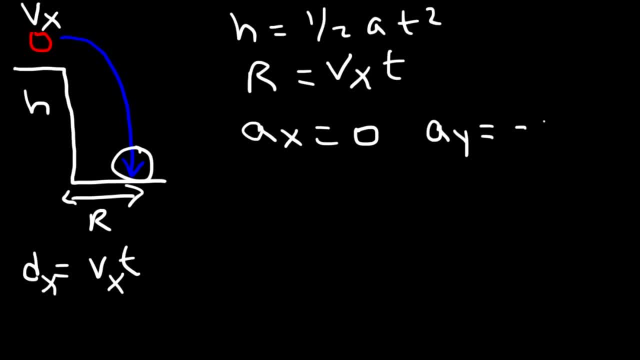 The acceleration in the y direction, that's the gravitational acceleration, it's negative 9.8.. And so vy changes. To calculate vy. we can use this equation: v final equals v initial plus at, But we're going to use it in the y direction. 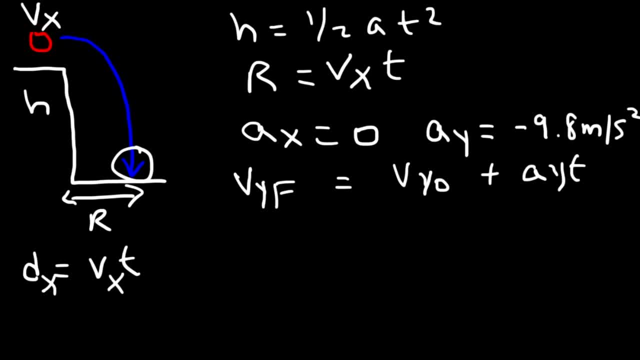 So we know that vy initial is 0.. At the top vy is always 0. So you can find vy final using this equation. Now, to find the speed of the ball just before it hits the ground, you need to use the. 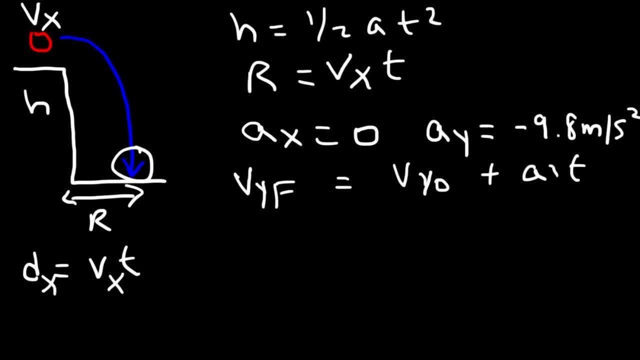 direction. So we know that vy initial is zero. At the top vy is always zero. So you can find vy final using this equation. Now, to find the speed of the ball just before it hits the ground, you need to use the horizontal velocity and the vertical velocity, And if. 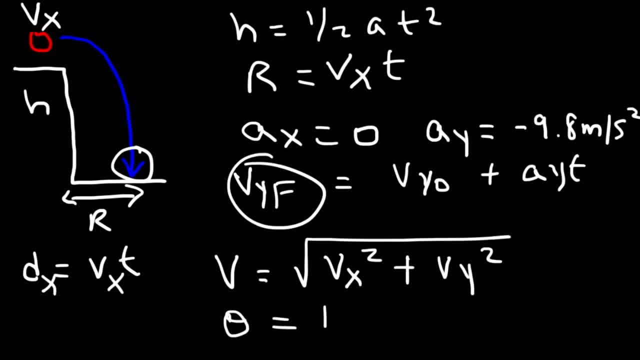 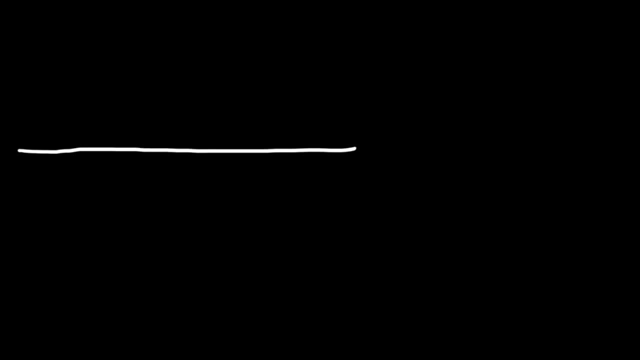 you need to find the angle. you can use this equation: It's inverse tangent vy divided by vx. Now, the second type of trajectory involves this type of fiction. So let's say, if we have a ball and we kick the ball from the ground, 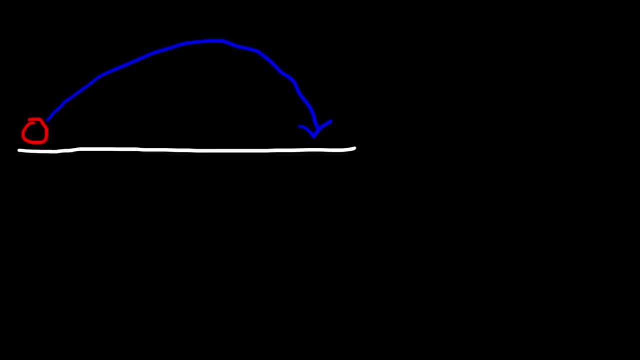 It goes up and then it goes down. So that ball is going to have an angle theta relative to the horizontal. it's going to be launched at a speed V. This is not Vx or Vy, this is V. Now let's draw. 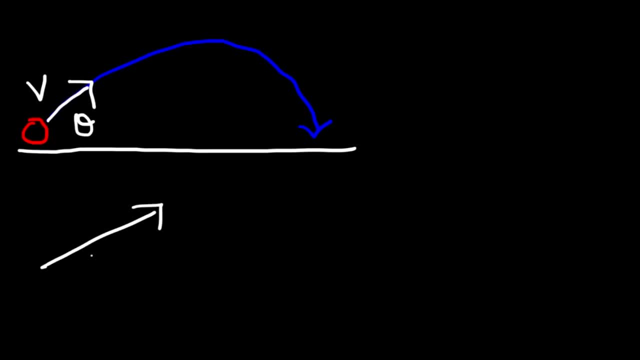 the vector V. So here's V and here's the angle theta. V has an x component and it has a y component. The x component is Vx, the y component is Vy. So Vx is equal to V cosine theta and Vy is equal to V sine theta. And V, as we mentioned before, is the square root. 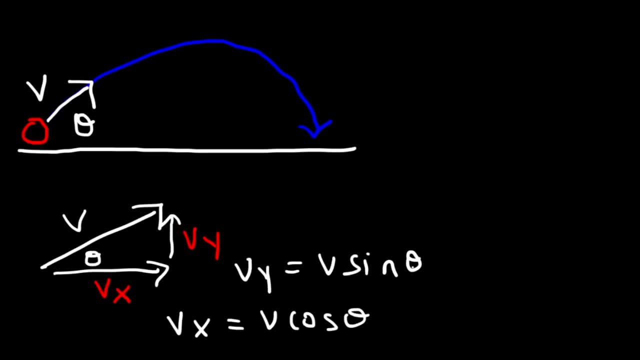 of Vx squared plus Vy squared And if you want to find theta, it's inverse tangent Vy over Vx. Now let's define this as point A, point B and point C. What is the equation that we need to calculate the time it takes to go from A to B or to reach the maximum? 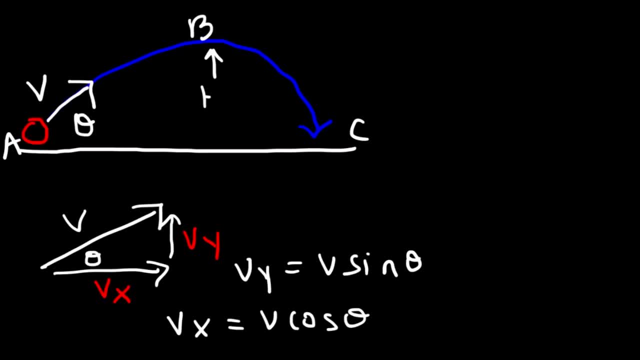 height, which is F. How long does it take to go from A to B? Now, to derive that equation, we need to start with this equation. V final equals V initial plus At, But we're going to use it in the y direction, So this is going to be Vy final. 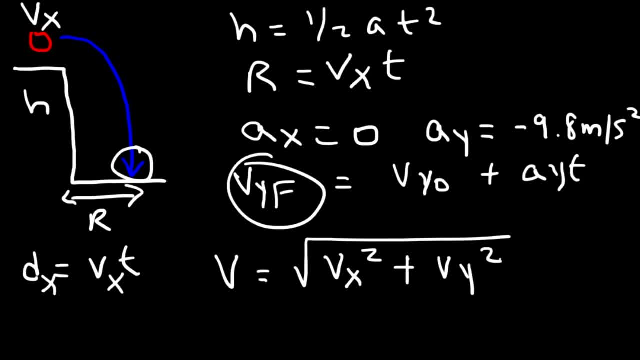 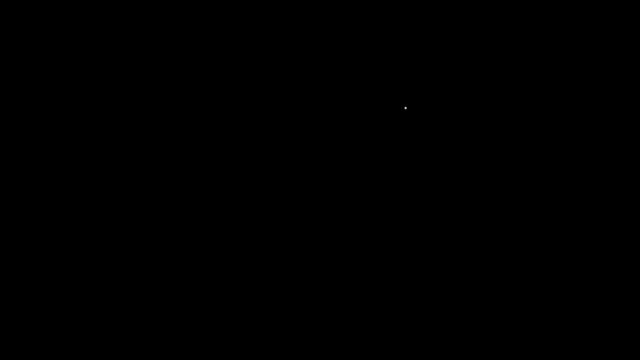 Horizontal Velocity and the Vertical Velocity. And if you need to find the angle, you can use this equation: It's inverse tangent vy divided by vx. Now, the second type of trajectory involves this type of fiction. So let's say, if we have a ball, 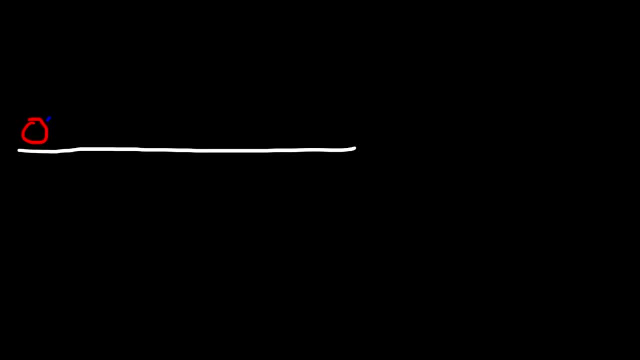 and we kick the ball from the ground. it goes up and then it goes down. So that ball is going to have an angle theta relative to the horizontal, and it's going to be launched at a speed v- This is not vx, or vy, this is v. 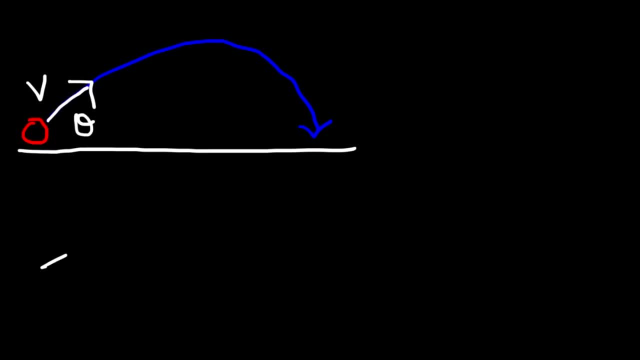 Now let's draw the vector v. So here's v and here's the angle theta v has an x component and it has a y component. The x component is vx, The y component is vy, So vx is equal to v cosine theta. 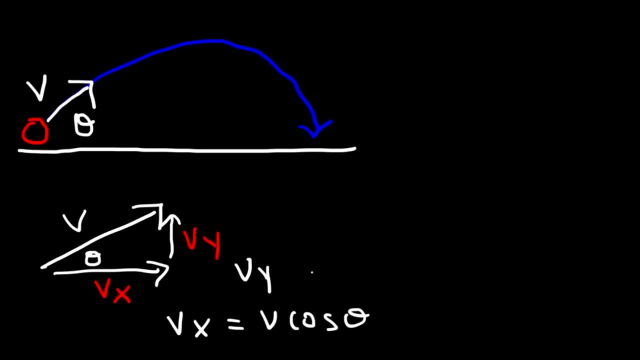 and vy is equal to v sine theta And v, as we mentioned before, is the square root of vx squared plus vy squared And if you want to find theta, it's inverse tangent: vy over vx. Now let's define this as point A, point B and point C. 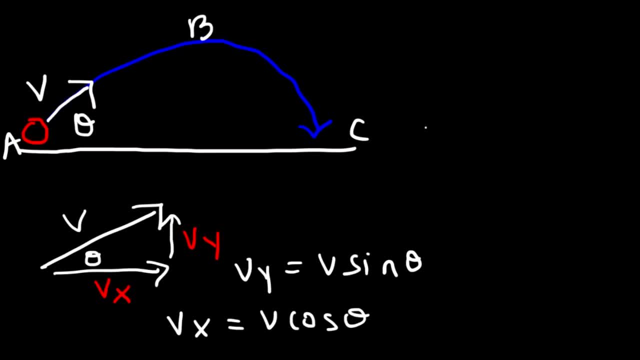 What is the equation? that we need to calculate the time it takes to go from A to B or to reach the maximum height which is at position B. How long does it take to go from A to B? Now to derive that equation? 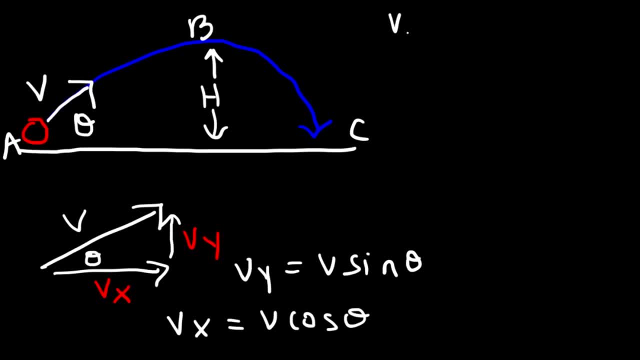 we need to start with this equation: v final equals v initial plus at, But we're going to use it in the y direction. So this is going to be: vy final equals, vy initial plus at, At the top, that is, at position B. 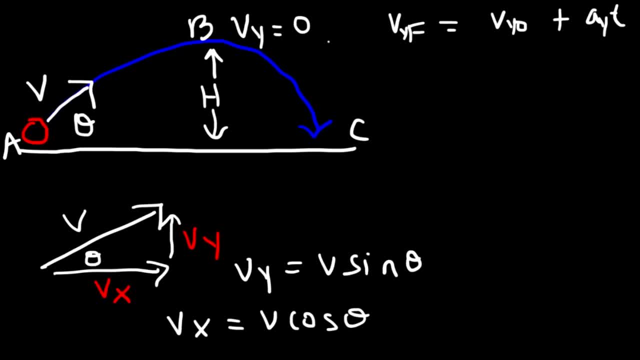 vy is always 0, because it's not going up anymore. So B is the final position, A is the initial position, So vy final is 0.. vy initial is basically v sine theta. as we wrote it in this equation. Acceleration in the y direction is basically g. 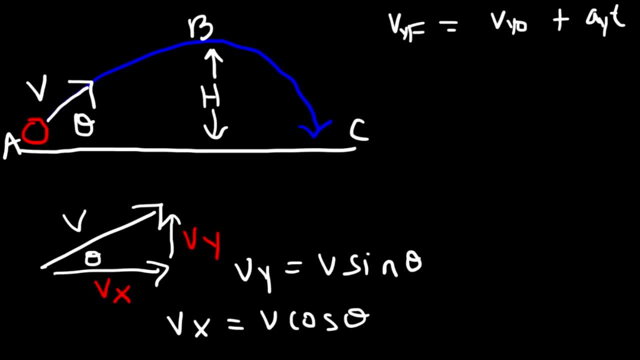 equals Vy initial plus At. At the top, that is, at position B, Vy is always zero because it's not going up anymore. So B is the final position. A is the initial position, So Vy final is zero. Vy initial is basically V sine theta, as we wrote it in this equation: Acceleration in the y direction. 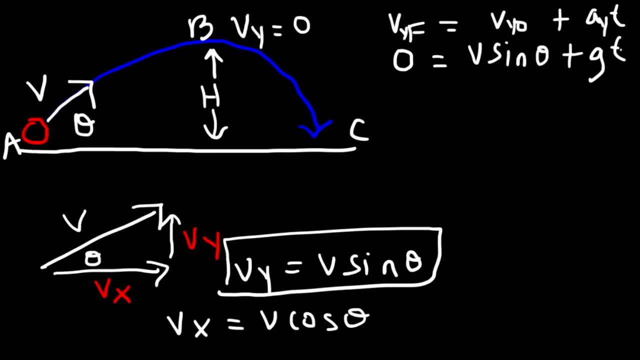 is basically G. So solving for T, we need to move this term to the other side. So negative V sine theta equal to gt, and dividing both sides by g, we can see that t is equal to v sine theta over g. so that's the time it takes to go from a to b. the time it takes to go from a to c. 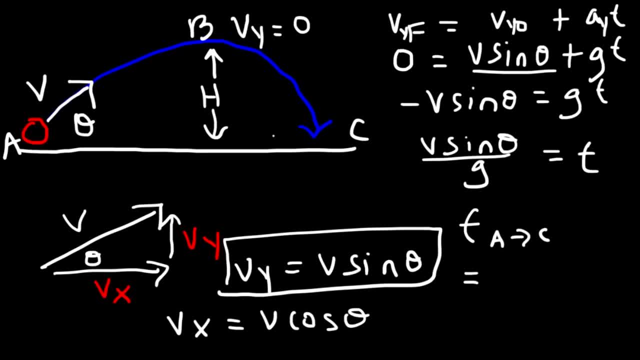 is twice the value. notice that the graph is symmetrical. so if it takes five seconds to go from a to b, it takes five seconds to go from b to c, and so to go from a to c it's 10 seconds. to the total time it's just 2 v sine theta, divided by g. if you're wondering what happened. 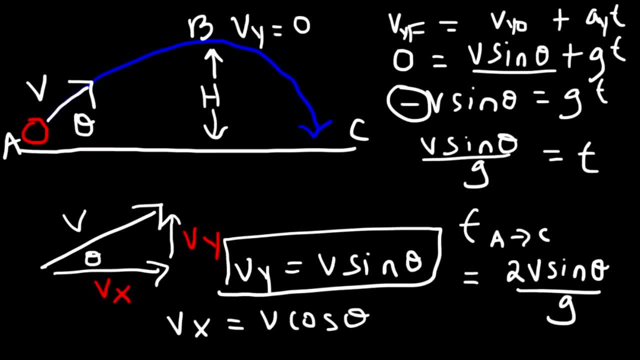 to the negative sign know that the g is negative 9.8, so it cancels with the negative sign. but if you plug in positive 9.8, you don't need the negative sign anymore either. case time is always positive, so so just make sure you report a positive value for time. now let's talk about 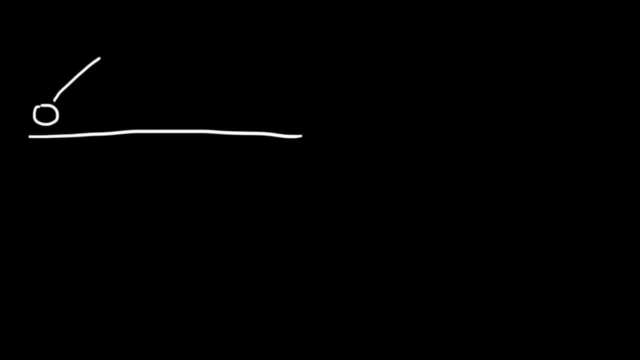 some other equations that relate to this shape. how can we derive an expression to calculate the maximum height between position a and position b, so going from a to b? let's use this particular kinematic equation: v final or vy final squared is equal to vy initial squared plus 2 times ay. 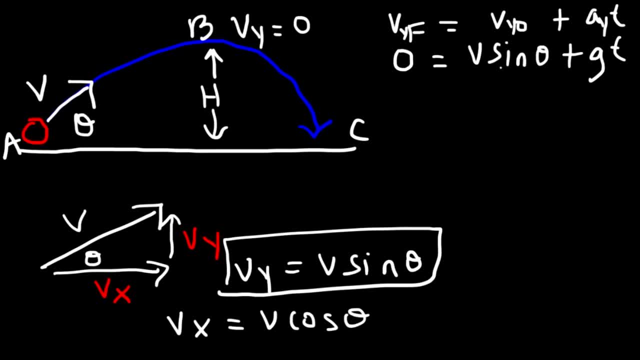 So solving for t, we need to move this term to the other side. So negative v sine theta is equal to gt, And dividing both sides by g, we can see that t is equal to v sine theta over g. So that's the time it takes to go from A to B. 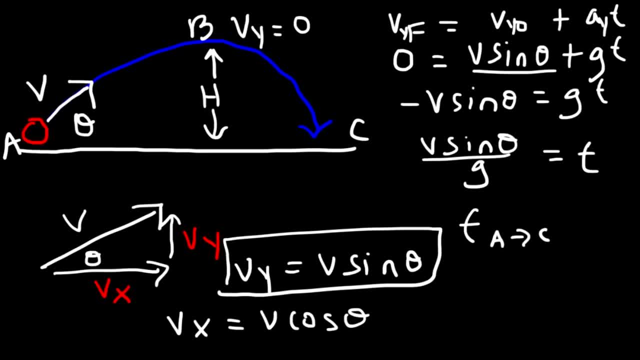 The time it takes to go from A to C is twice the value. Notice that the graph is symmetrical. So if it takes 5 seconds to go from A to B, it takes 5 seconds to go from B to C, And so to go from A to C it's 10 seconds. 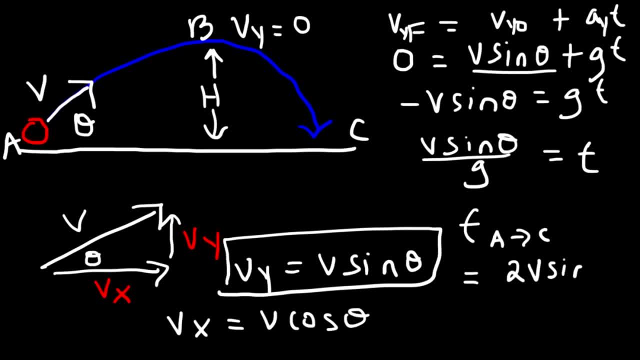 So the total time is just 2v sine theta divided by g. If you're wondering what happened to the negative sign, know that g is negative 9.8, so it cancels with the negative sign, But if you plug in positive 9.8,. 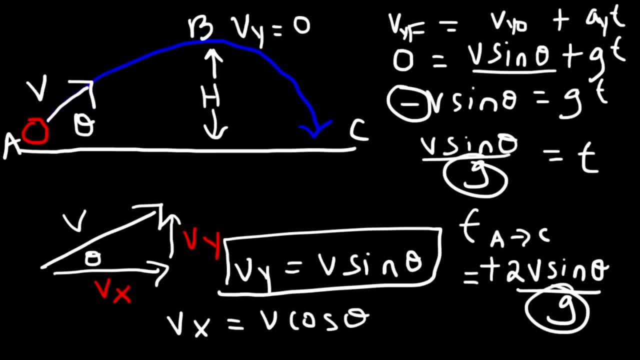 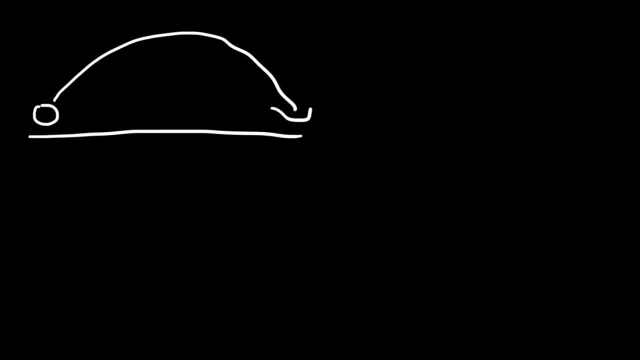 you don't need the negative sign anymore. Either case time is always positive, So just make sure you report a positive value for time. Now let's talk about some other equations that relate to this shape. How can we derive an expression to calculate the maximum height? 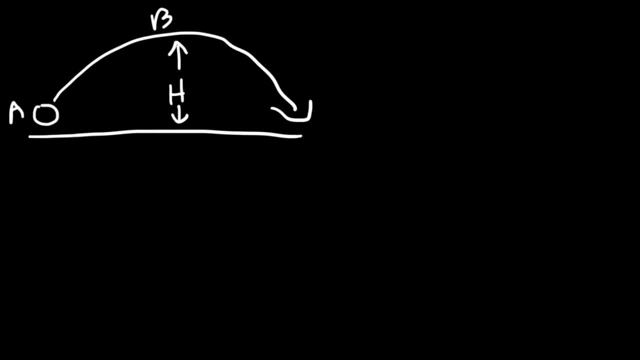 between position A and position B. So, going from A to B, let's use this particular kinematic equation: v final or vy final squared is equal to vy initial squared plus 2 times ay times dy. So you've seen it as v final squared. 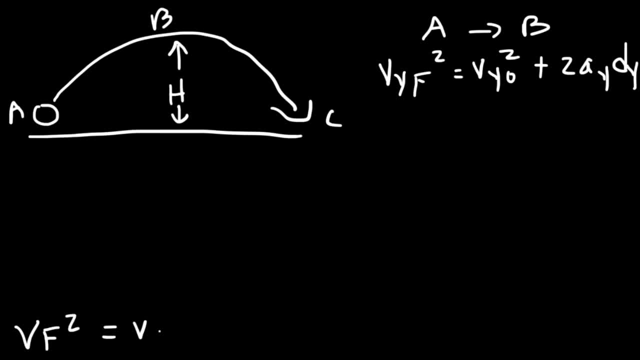 equals v, initial squared plus 2ad. I simply added the subscript y to it because the height is in the y direction. Now, at the top, vy is equal to 0. So position B is equal to 0.. v is the final position. 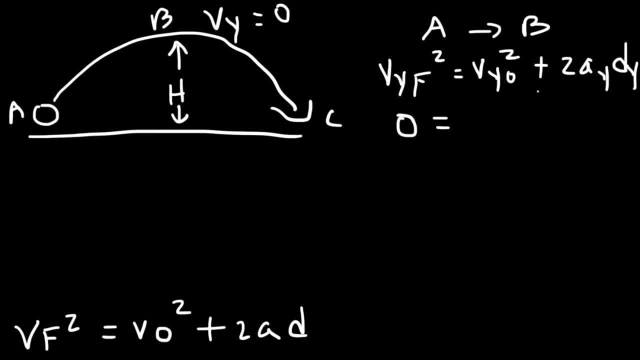 So vy final is 0.. vy initial, we know that vy is v sine theta. So vy squared is v sine theta squared, And of course we have plus 2 times. the acceleration in the y direction is g. the displacement in the y direction 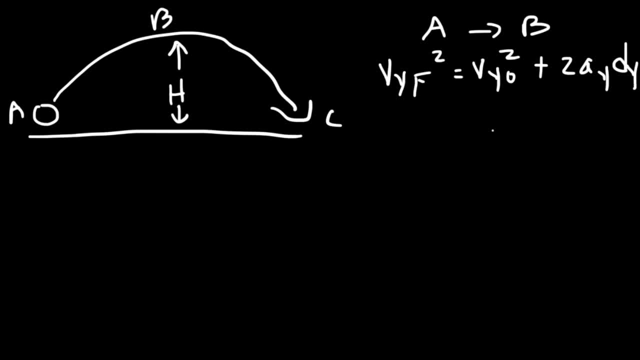 times dy. so you've seen as v final squared equals v initial squared plus 2 a d. i simply added the subscript y to it because the height is in the y direction. now, at the top, vy is equal to 0.. so position b is the final position. so vy final is 0.. vy initial. we know that vy is v sine theta. 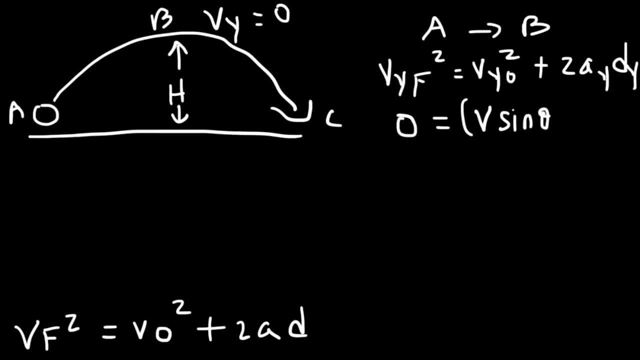 so vy squared is v sine theta squared, and of course we have plus two times. the acceleration in the y direction is g. the displacement in the y direction is the same as the height, so we can put h at this point. so let's move this term to the left. so negative: v squared sine square. 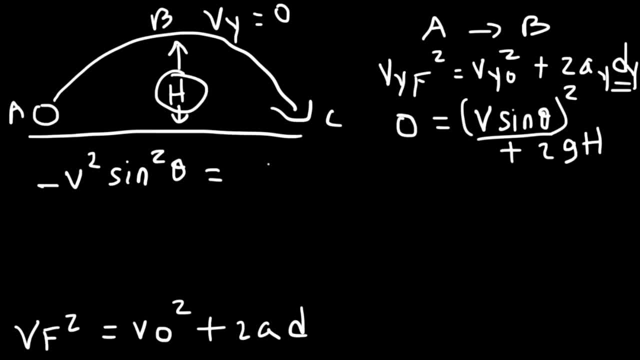 theta, if you distribute the two, is equal to 2gh. now let's divide by 2g. so the maximum height, if we ignore the negative sign, is v squared sine, squared theta over 2g. so that's how you can find the height if you have the angle theta. 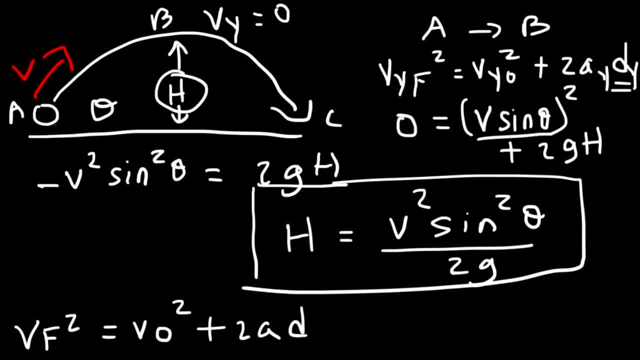 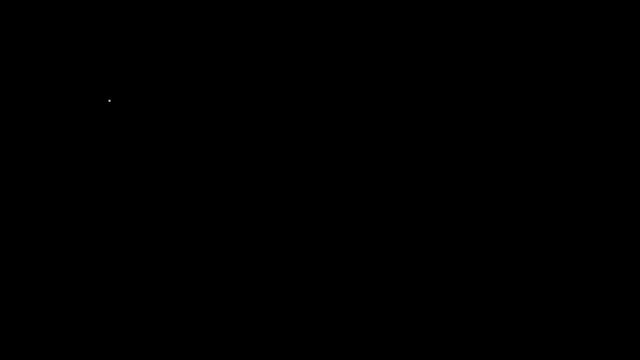 and the velocity, not vx of vy, but the velocity v. now what equation can we come up with in order to calculate the range? how can we derive an equation to find the range of the graph? what equation would you use? the range is the horizontal distance or the horizontal displacement of the ball. now we said that the range is equal to vxt. 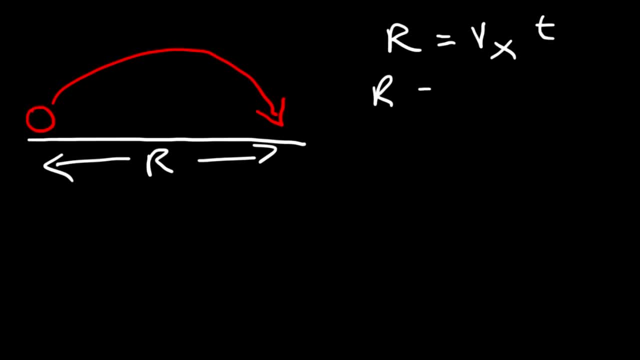 and you can find vx by using the fact that vx is v cosine theta. now the range is the horizontal displacement from points a to c. so what is the time from point a to c? as you mentioned earlier in this video, the time it takes for the ball to go from a to c is equal to 2v sine theta. 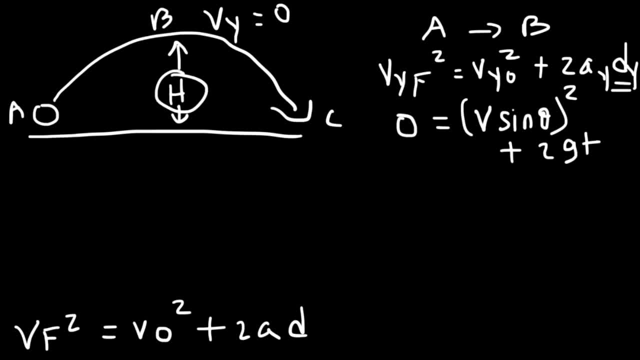 is the same as the height, So we can put h at this point. So let's move this term to the left. So negative v squared sine, squared theta, if you distribute the two, is equal to 2gh. So now let's divide by 2g. 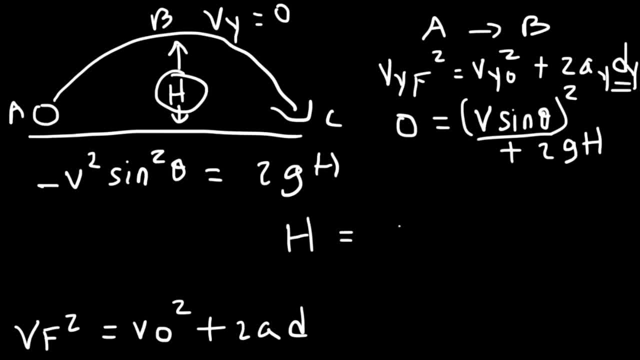 So the maximum height, if we ignore the negative sign, is v squared sine squared theta over 2g. So that's how you can find the height if you have the angle theta and the velocity, Not vx or vy, but the velocity v. 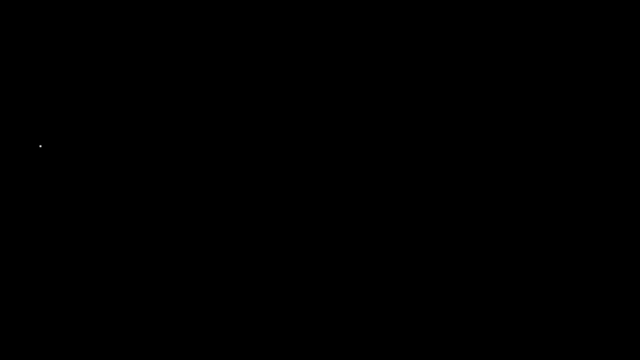 Now, what equation can we come up with in order to calculate the range? How can we derive an equation to find the range of the graph? What equation would you use? The range is the horizontal distance or the horizontal displacement of the ball. Now, we said that the range 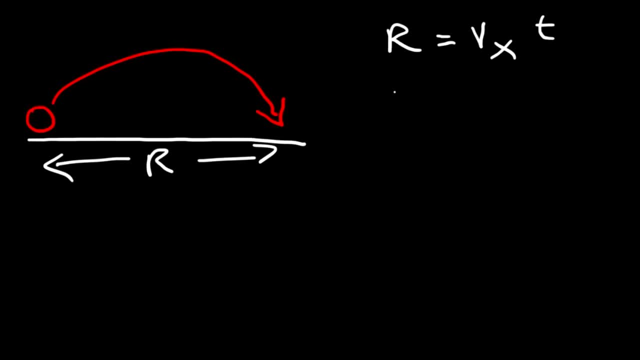 is equal to vxt And you can find vx by using the fact that vx is v cosine theta. Now the range is the horizontal displacement from points A to C. So what is the time? from point A to C, As we mentioned earlier in this video, 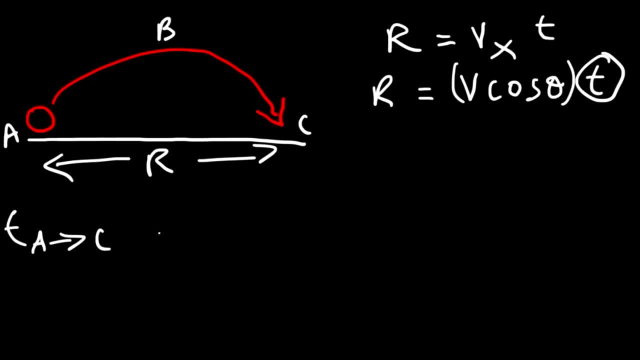 the time it takes for the ball to go from A to C is equal to 2v sine theta divided by g. So we have v cosine theta and we're going to replace t with 2v sine theta over g. Now v times v. 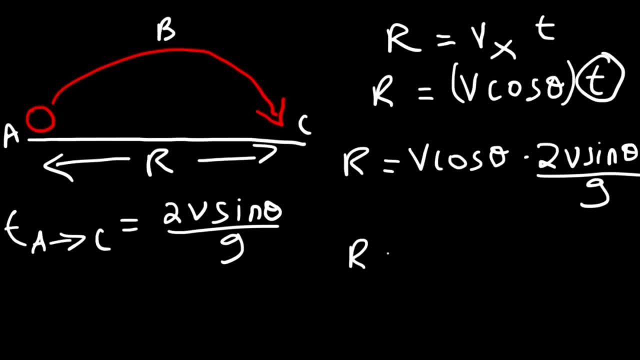 is basically v squared, So we have v squared times 2 sine theta, cosine theta divided by g. Now there's something called a double angle formula in trigonometry, And here it is: Sine 2 theta is equal to 2 sine theta. 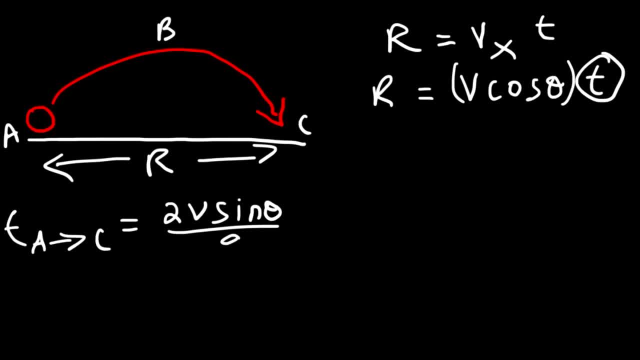 sine theta divided by G. so we have V cosine theta and we're gonna replace T with 2 V sine theta over G. now V times V is basically V squared. so we have V squared times 2 sine theta, cosine theta divided by G. now there's something. 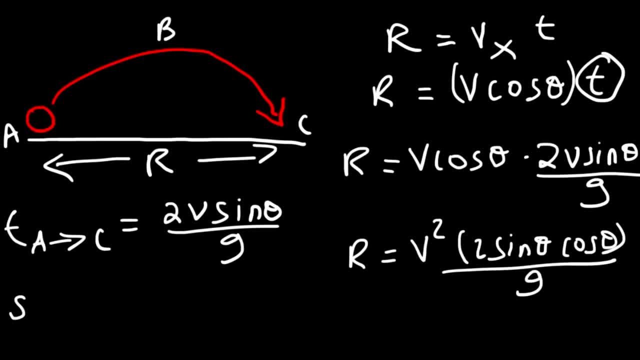 called a double angle formula in trigonometry, and here it is. sine 2 theta is equal to 2 sine theta cosine theta, so therefore we can replace the expression 2 sine theta cosine theta with sine 2 theta, And so therefore the range 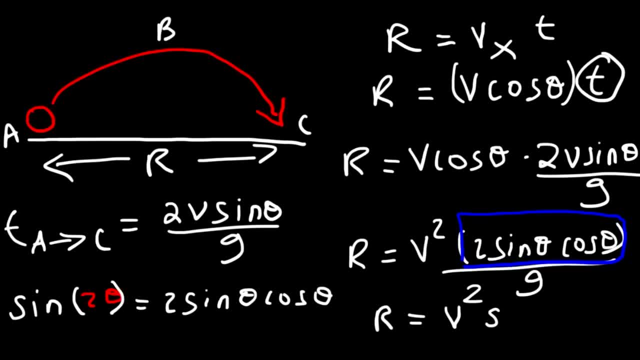 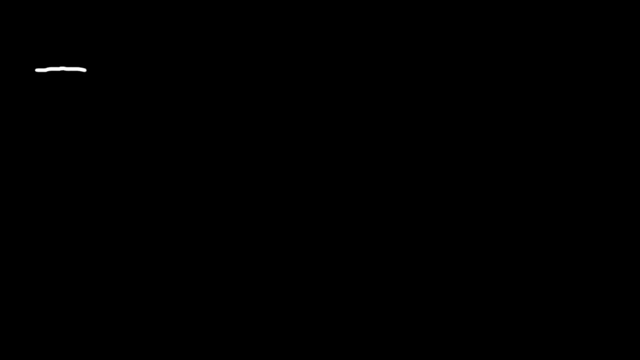 is V squared sine 2, theta divided by G. So that's how you can derive an equation for the range if you have this type of trajectory. Now the third type of trajectory that you're going to see involves a ball being launched at an angle from a cliff. 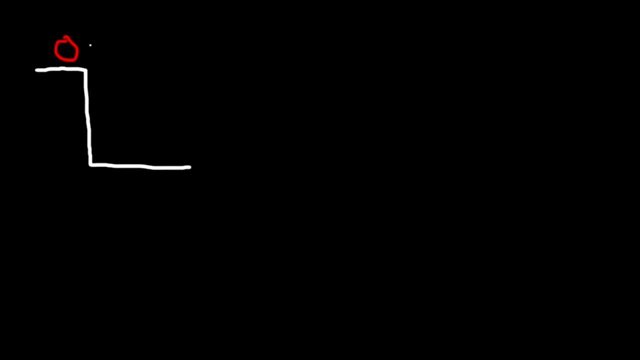 or from some elevated position above ground level. So it's going to go up and then it's going to go down. So H is the height of the cliff and R, once again, is the range of the ball. Let's call this position A. 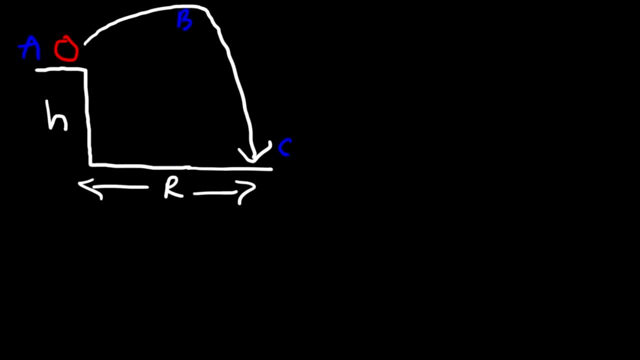 position B and position C. So one of the first type of questions that you might find with this type of problem is calculating the time it takes to hit the ground going from A to C. Now, this graph is not the same as this trajectory. 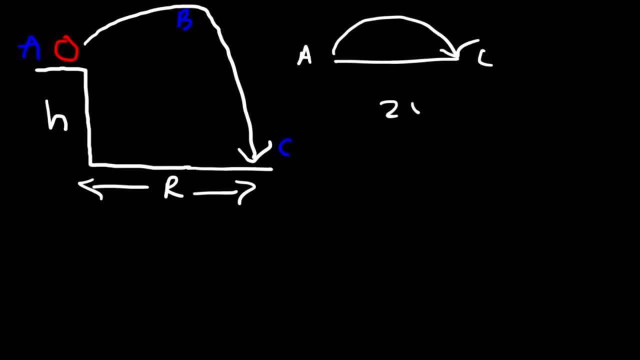 where the time it takes to go from A to C is 2V, sine theta, over G. If you use this equation, that'll give you the time it takes to get to this position, which is symmetrical to A. so don't do it, it's not going to work. 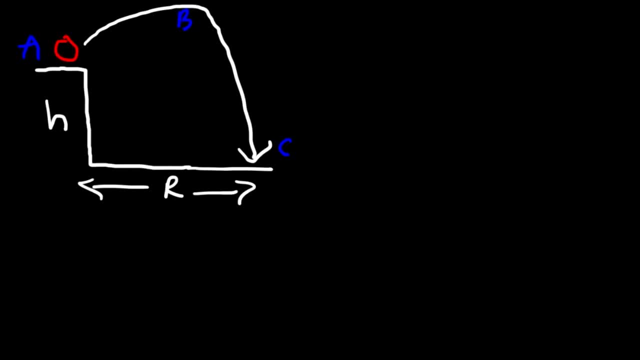 So therefore, we need to do something else. It turns out that there's another way to calculate the time. I'm going to show you two ways, so please be patient. Let's start with this equation. Displacement is equal to V. initial T. 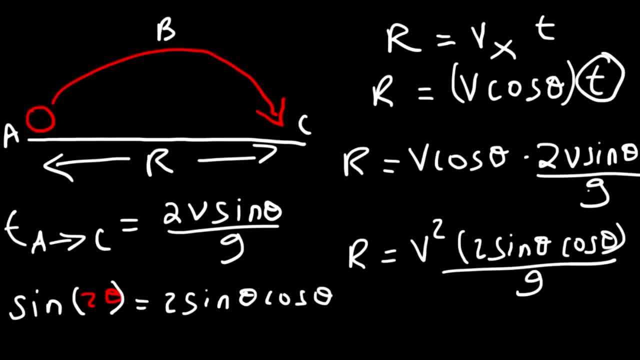 cosine theta. So therefore we can replace the expression 2 sine theta cosine theta with sine 2 theta, And so therefore the range is v squared sine 2 theta divided by g. So that's how you can derive an equation for the range. 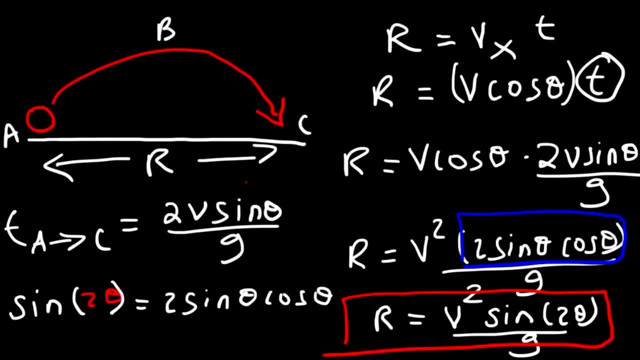 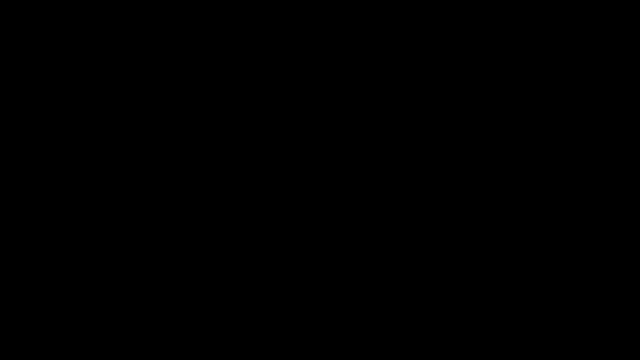 If you have this type of trajectory. Now, the third type of trajectory that you're going to see involves a ball being launched at an angle, from a cliff Or from some elevated position above ground level. So it's going to go up and then it's going to go down. 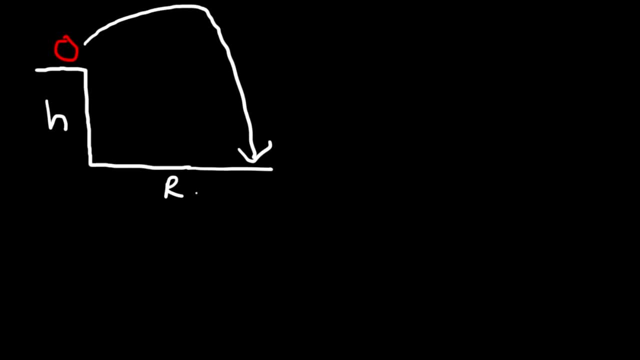 So h is the height of the cliff and r, once again, is the range of the ball. Let's call this position a, position b and position c. So one of the first type of questions that you might find with this type of problem. 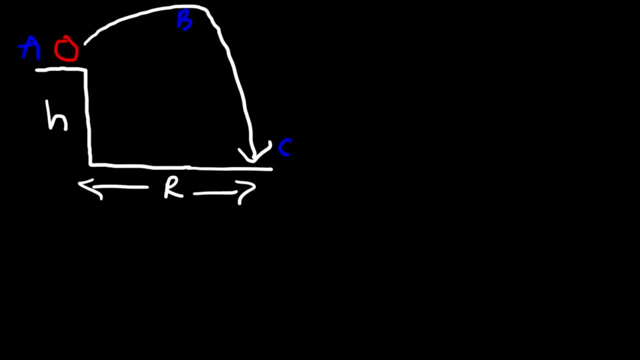 is calculating the time it takes to hit the ground going from a to c. Now, this graph is not the same as this trajectory, where the time it takes to go from a to c is 2 sine theta over g, If you use this equation. 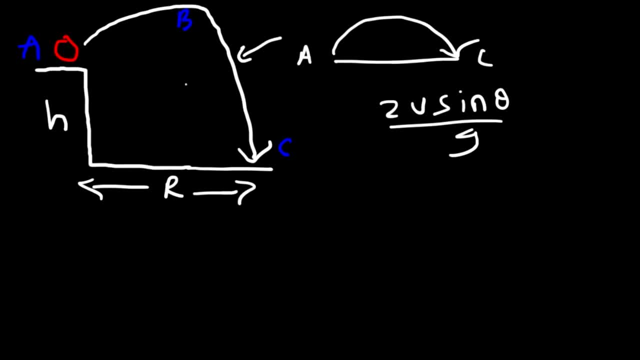 that'll give you the time it takes to get to this position, Which is symmetrical to a. so don't do it. it's not going to work. So therefore we need to do something else. It turns out that there's another way to calculate the time. 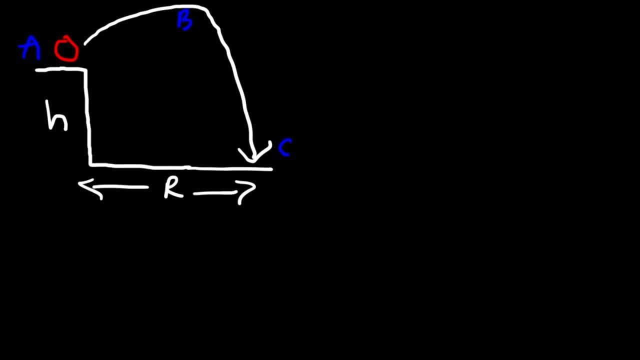 I'm going to show you two ways, so please be patient. Let's start with this equation. Displacement is equal to v, initial t plus 1, half a t squared, But we're going to apply it in the y direction. Displacement in the y direction. 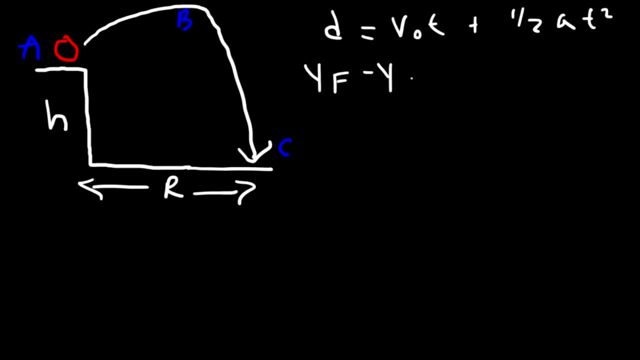 is the difference between the final position minus the initial position And then v initial. but in the y direction is v y initial Acceleration in the y direction is basically 9.8 or g. So moving this term to the other side, perhaps you've seen. 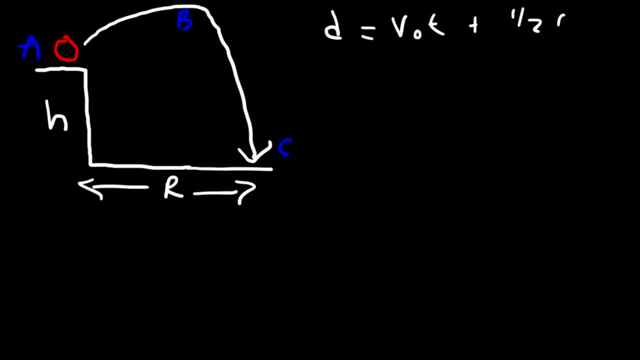 plus 1 half A T squared. But we're going to apply it in the Y direction. Displacement in the Y direction is the difference between the final position minus the initial position And then V initial, but in the Y direction is VY initial. 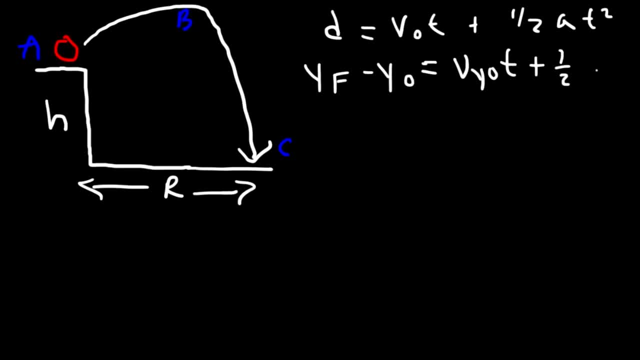 Acceleration in the Y direction is basically 9.8 or G. So moving this term to the other side, perhaps you've seen this equation: Y final equals Y initial. Y initial is basically the height of the cliff plus VY initial, T. 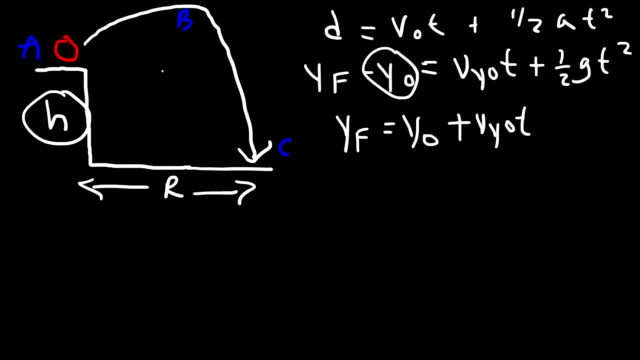 Remember VY initial is V sine theta. Theta is the angle above the horizontal plus 1 half G T squared. Now, to find the time it takes to hit the ground, you need to realize that the position, the Y value at ground level is 0.. 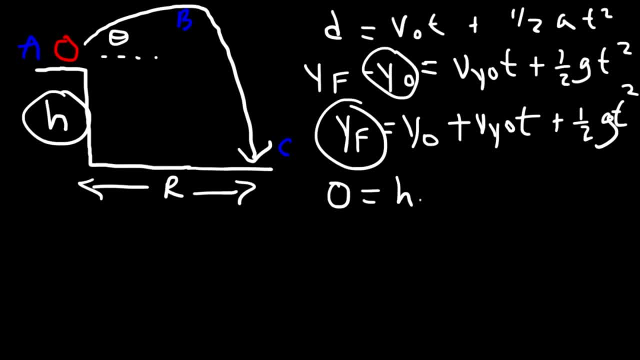 So if you replace it with 0, replace Y initial with H, replace VY initial with V sine theta, you now have everything you need to solve for T. You know what G is. However, you need to use a quadratic equation. 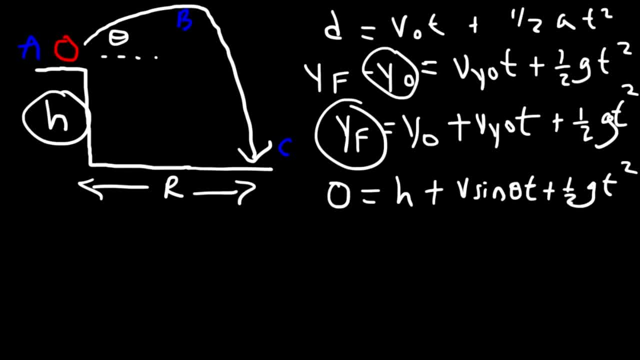 You want to make sure everything's on one side and on the other side you have a 0. So, using the quadratic formula, T is equal to negative B plus or minus square root, B squared minus 4AC divided by 2A. So let's say: if you get an equation, 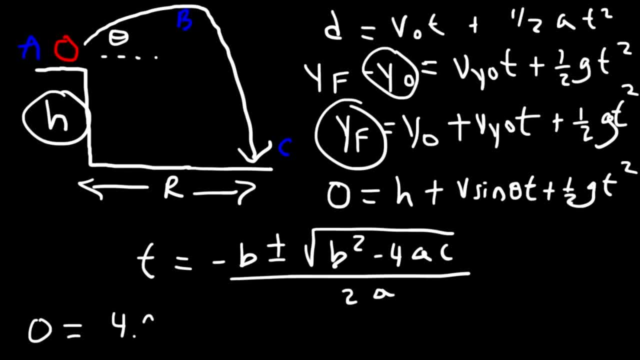 that looks like this, and you put it in standard form: 4.9 T squared Plus 8T plus 100 or something like that In this case. well, actually this is going to be negative 4.9 T squared. You got to make sure you plug in negative 9.8 for G. 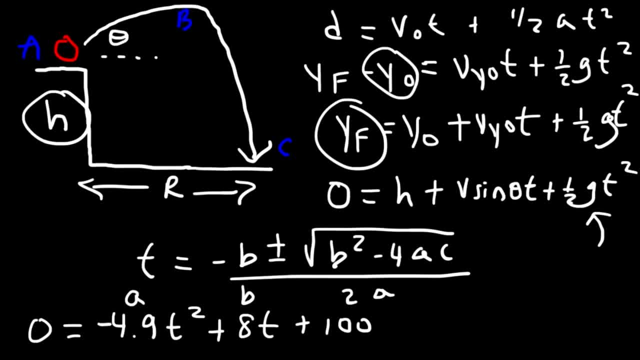 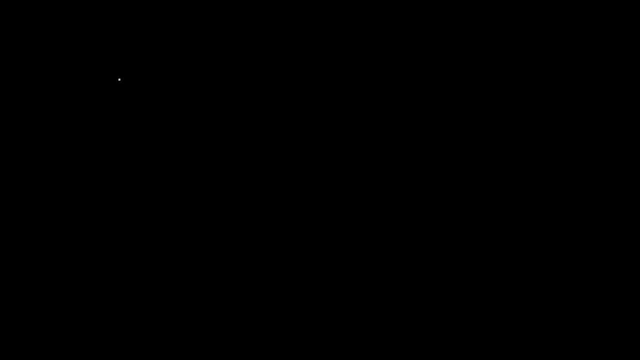 A is negative 4.9.. B is 8.. C is 100.. And then just plug it into this formula and you should get the answer. Now let's go back To the same trajectory. Now, what's another way in which we can calculate the time? 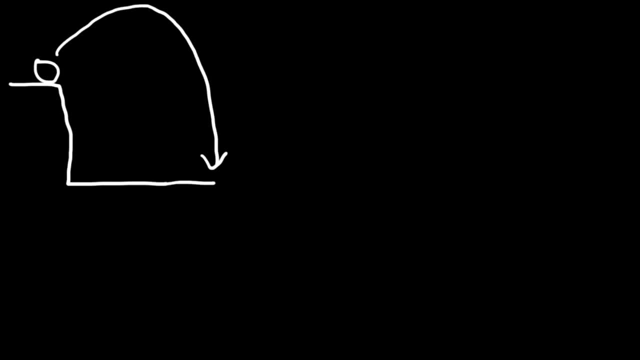 That is the time it takes to hit the ground To go from position A to position C. Is there a way in which we can get the same answer without using the quadratic equation? It turns out that there is To go from A to B. 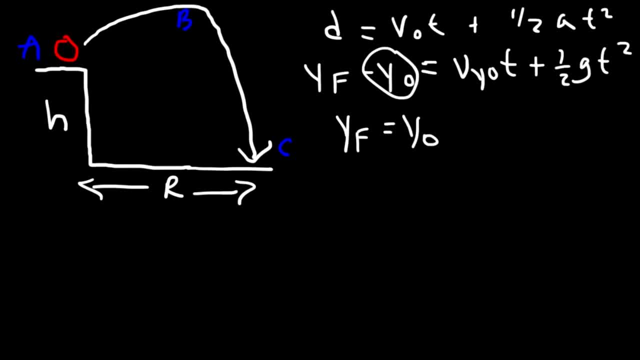 this equation, y final equals y initial. y initial is basically the height of the cliff plus v y initial. t Remember, v y initial is v sine theta. Theta is the angle above the horizontal Plus 1 half g t squared. Now to find the time. 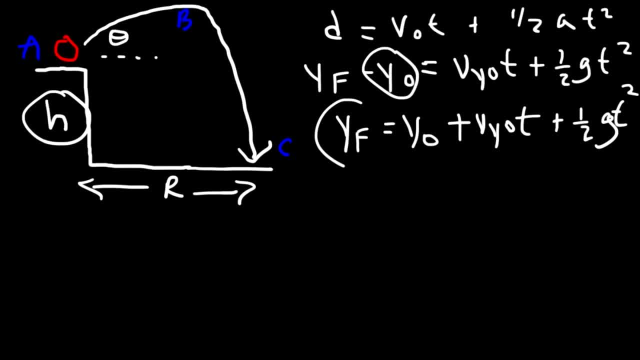 it takes to hit the ground. you need to realize that the position, the y value at ground level is 0. So if you replace it with 0,, replace y initial with h, replace v y initial with v sine theta, you now have everything you need. 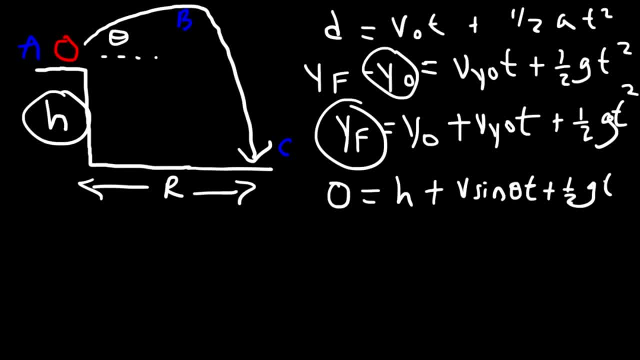 to solve for t, You know what g is. However, you need to use a quadratic equation. You want to make sure everything is on one side, and on the other side you have 0. So using the quadratic formula, t is equal to negative b. 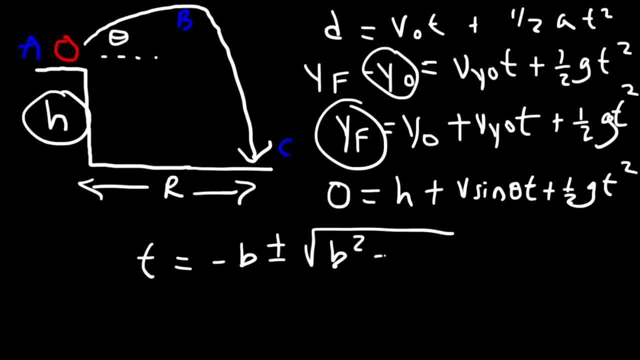 plus or minus b squared minus 4ac divided by 2a. So let's say, if you get an equation that looks like this and you put it in standard form, 4.9 t squared plus 8t plus 100, or something like that. 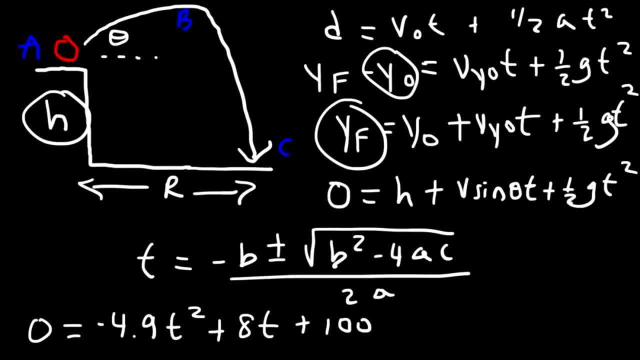 In this case. well, actually this is going to be negative 4.9 t squared. You got to make sure you plug in 9.8 for g a is negative 4.9, b is 8, c is 100.. 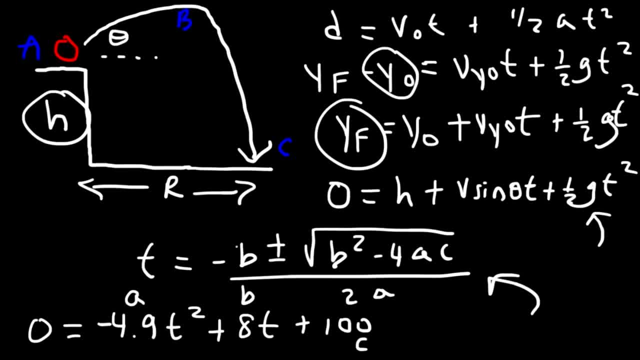 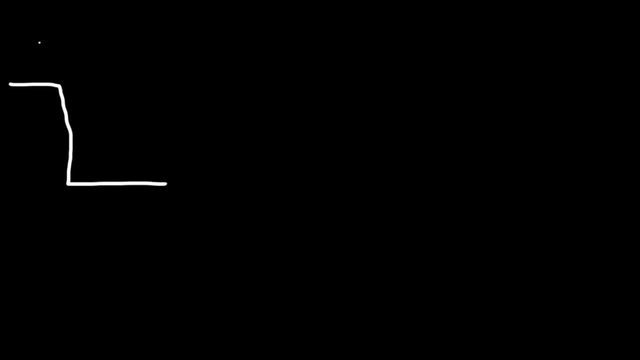 And then just plug it into this formula and you should get the answer. Now let's go back to the same trajectory. Now, what's another way in which we can calculate the time, That is, the time it takes to hit the ground To go from position a? 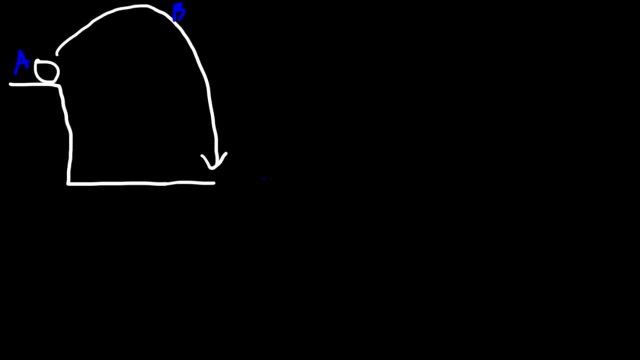 to position c. Is there a way in which we can get the same answer without using the quadratic equation? It turns out that there is To go from a to b. notice that it's the same as this trajectory- So we can use the equation that we used in that trajectory. 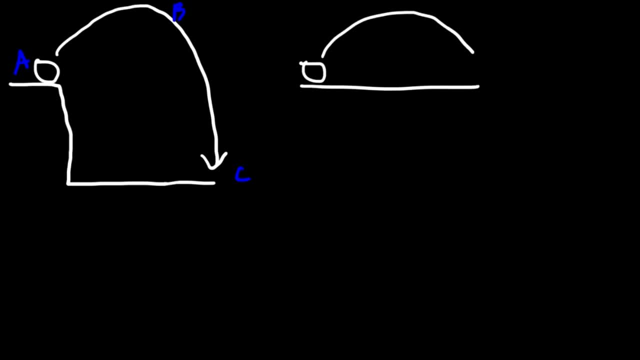 notice that it's the same as this trajectory, So we can use the equation that we used in that trajectory. The time it takes to go from A to B is simply V sine theta divided by G, And typically in this problem you'll be given V. 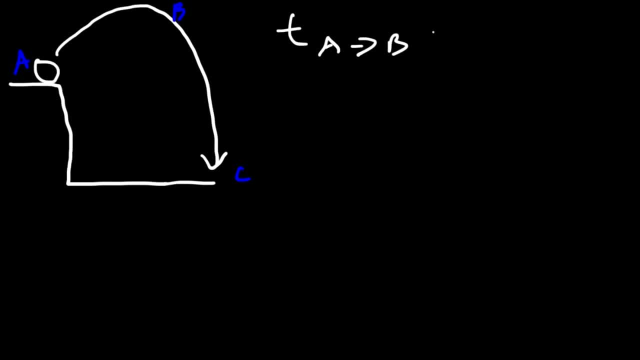 That is just the speed of the ball And you're going to be given theta- The angle of the ball. And you're going to be given theta- The angle of the ball. And you're going to be given theta- The angle of the ball. 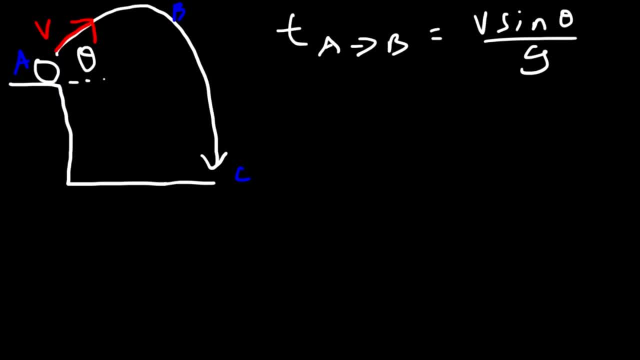 The angle of the ball. The angle of the ball, The angle relative to the horizontal, The angle relative to the horizontal. Now, how can we find the time it takes to go from B to C? Now, how can we find the time it takes to go from B to C? 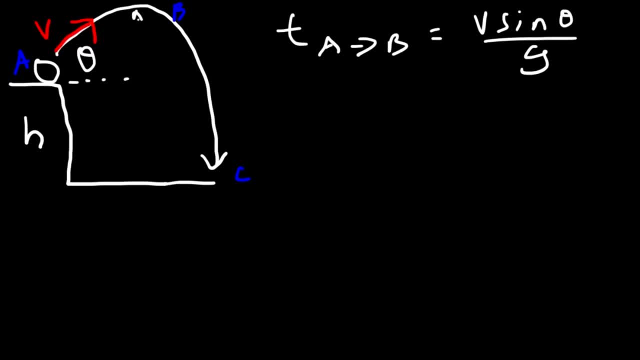 Well, in order to do that, you need to find the height between positions A and position B, between positions A and position B. To find that height, it's going to be equal to V squared sine squared, and I believe it was over 2G. 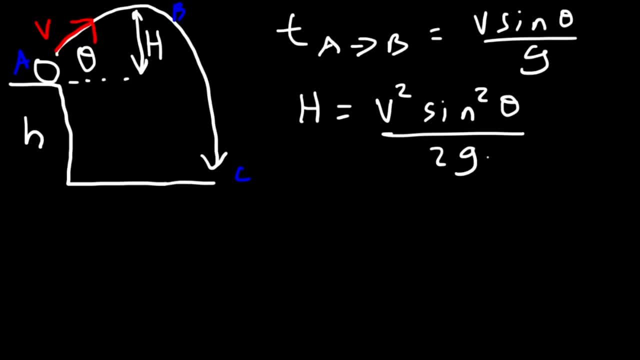 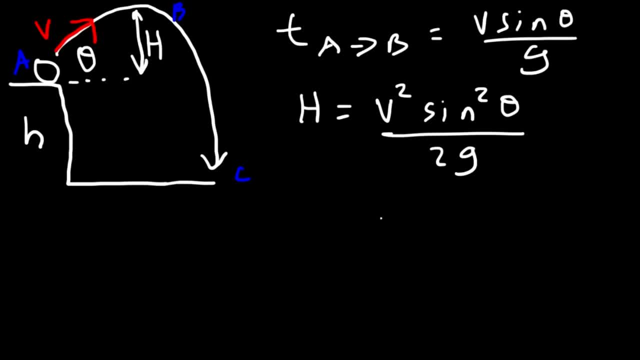 The total height from B to C. we can use that to find the time. Now you've seen this equation. h is equal to 1, half at squared, But in this particular situation between B and C, h it's really the sum. 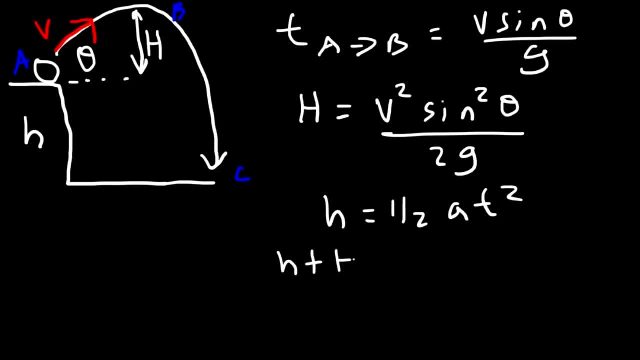 of h plus capital H, So that's the total height from B to C And that's equal to 1 half times t squared. So basically, if you rearrange the equation, t going from B to C is going to be- let's call this, y max. 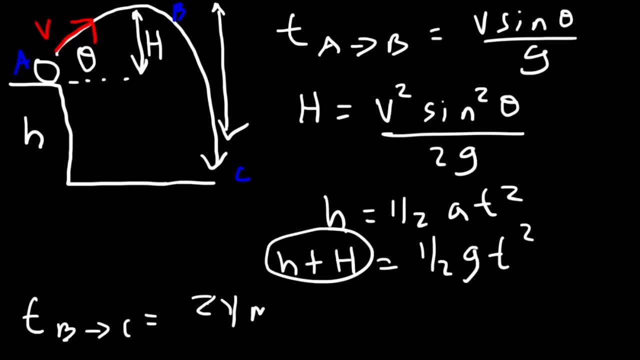 So 2 times y max, divided by G squared root, That's going to give you the time it takes to go from B to C. So the total time is simply the sum of these two values, And that's how you can avoid using the quadratic formula if you don't want to. 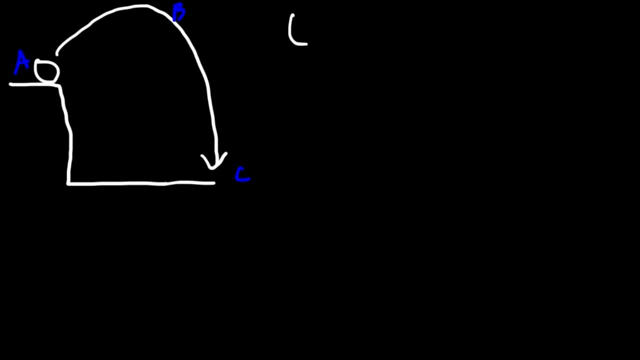 The time it takes to go from a to b is simply v sine theta divided by g, And typically in this problem you'll be given v, That is just the speed of the ball, And you're going to be given theta, The angle relative. 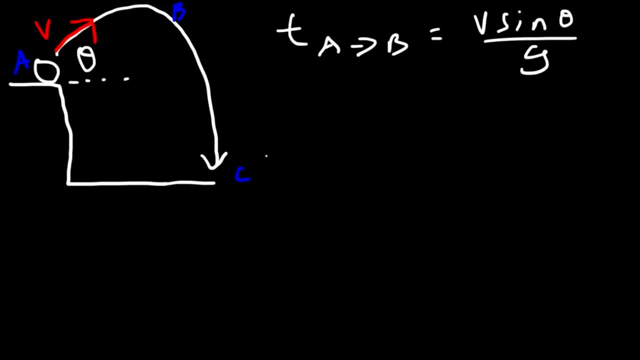 to the horizontal. Now, how can we find the time it takes to go from b to c? Well, in order to do that, you need to find the height between positions a and position b. To find that height, it's going to be equal to. 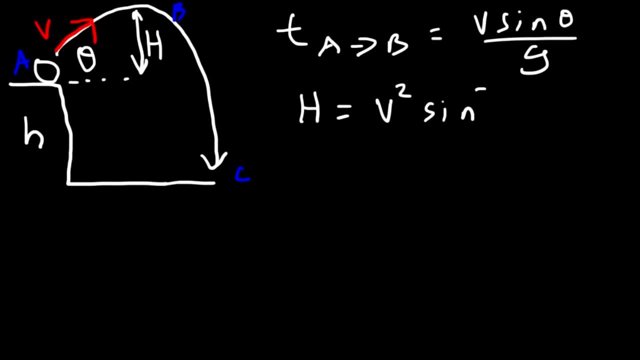 v squared sine squared, and I believe it was over 2g, if I'm not mistaken. I believe that's the equation. Once you get the height, then the total height, which let's call the total height y max, the total height from b to c. 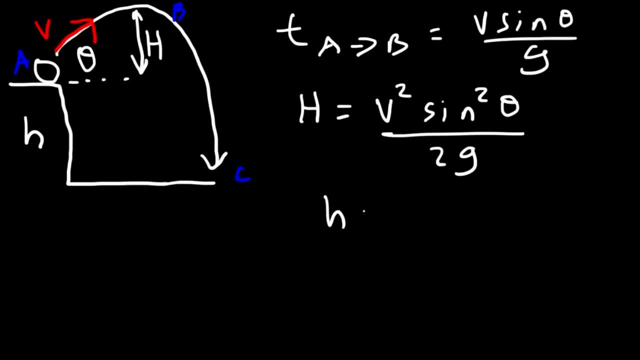 we can use that to find the time. Now. you've seen this equation: h is equal to 1, half a t squared. But in this particular situation between b and c, h is really the sum of h plus capital H, So that's the total height. 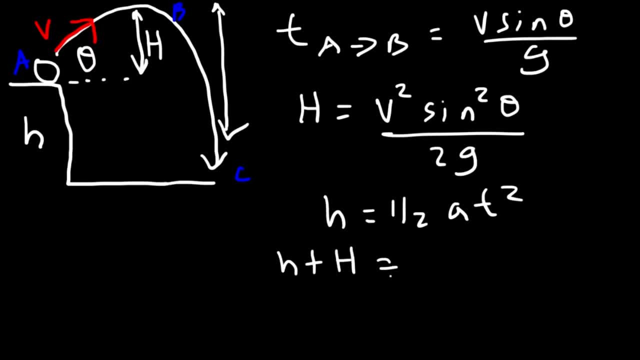 from b to c And that's equal to 1 half a, which is the same as g times t squared. So basically, if you rearrange the equation, t going from b to c is going to be- let's call this- y max, So 2. 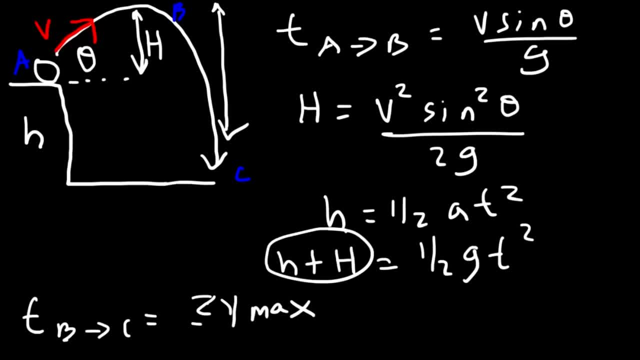 times y max divided by g square root. That's going to give you the time it takes to go from b to c. So the total time is simply the sum of these two values, And that's how you can avoid using the quadratic formula if you don't want to. 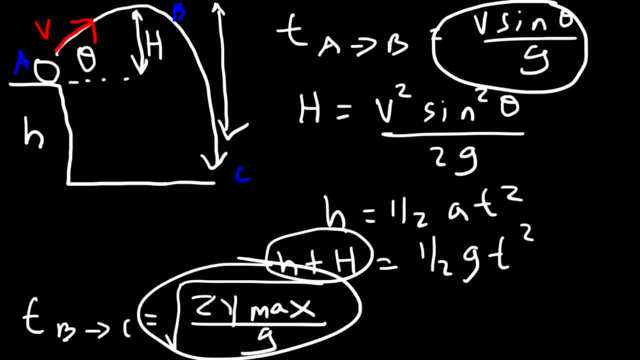 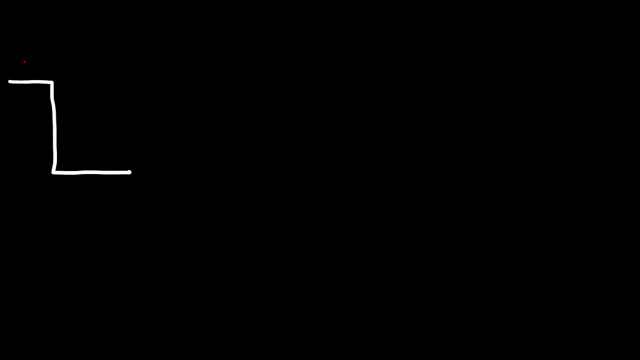 Now, how can we find a range? What equation would you use to calculate the range of the ball? To find a range, use this equation v x t For this trajectory. do not use the equation v x t For this trajectory. do not use the equation. 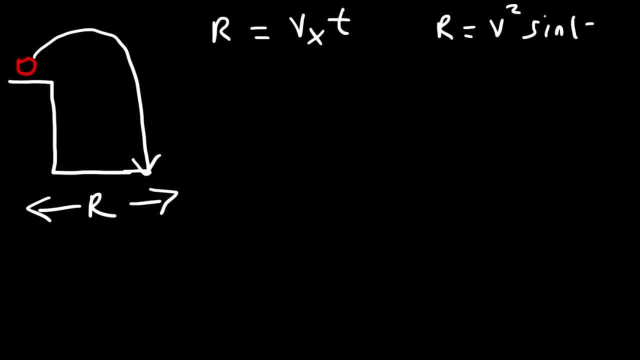 v squared sine 2 theta over g. Only use this equation if you have a symmetrical trajectory. This is the only time you should use this equation. Otherwise, if you use it for this problem, you're going to get the range between these two points. 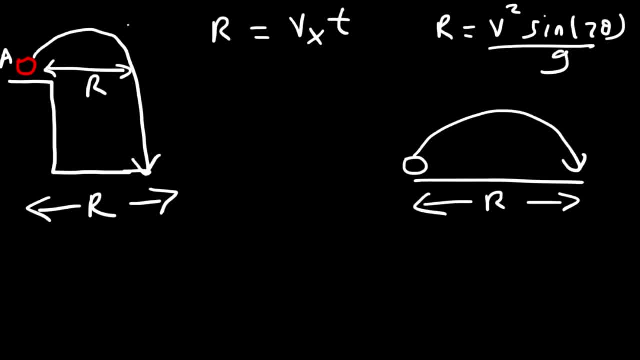 Let's call this point a and point d. You're going to get the range between those two points and you don't want that. So to find a range for this type of trajectory, use the equation v x times t. Now keep in mind v- x. 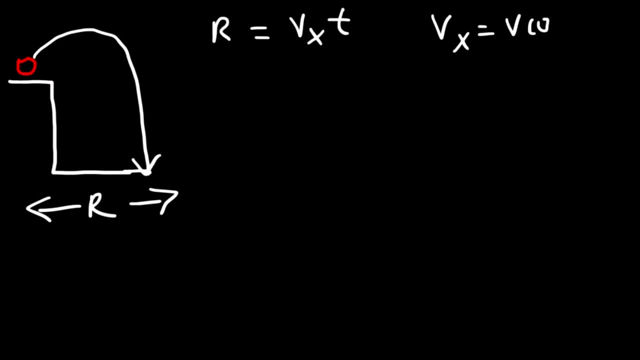 is equal to v cosine theta, So the range is simply v times cosine theta times t. You can use this form of the equation if you want to, But you need to find the time it takes to go from a to c before you can use it, Which. 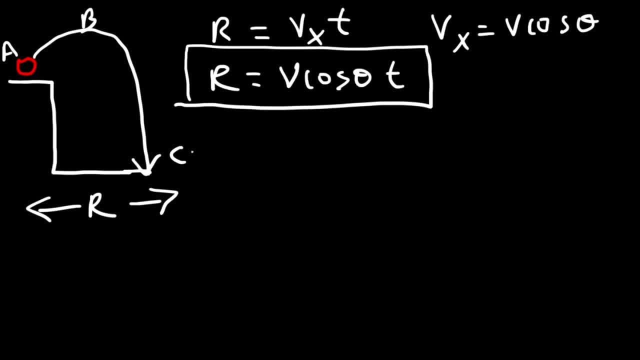 using the last two equations you can get that answer now. So that's all you need to do to find the range Now. sometimes you might be asked to find the speed of the ball just before it hits the ground. So first you need to realize that v- x is constant. 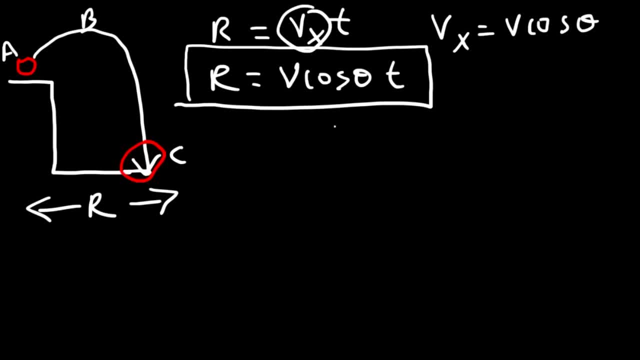 So whatever v x you have here is going to be the same at point c, At point a, point b and point c, v x is the same. So let me make sure I write that v x is constant. It does not change. So whatever. 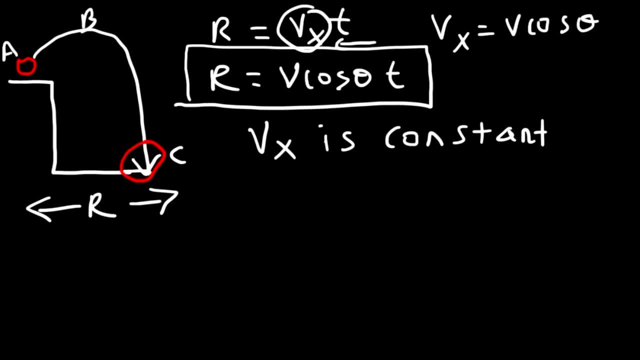 v, x you have here. just we're going to use that to find the final speed of the ball just before it hits the ground. Now, just like last time we mentioned earlier in this video, we've got to find the vertical velocity as well using this equation. 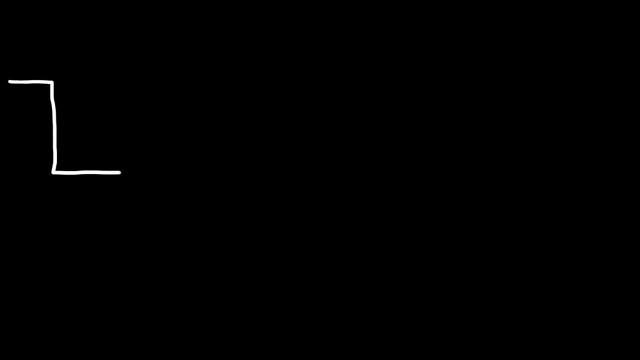 Now, how can we find a range? What equation would you use to calculate the range of the ball? To find a range, use this equation: v x, t For this trajectory. do not use the equation v squared sine 2 theta over G. Only use 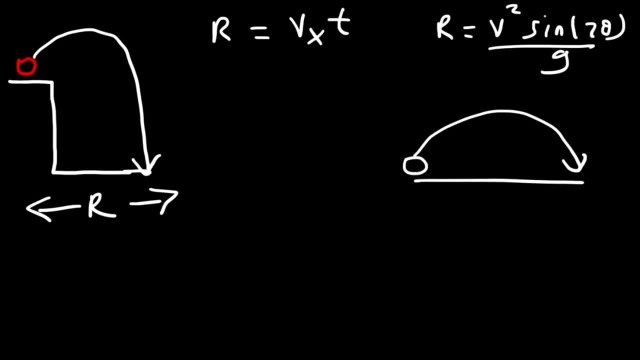 this equation. if you have a symmetrical trajectory, This is the only time you should use this equation. Otherwise, if you use it for this problem, you're going to get the range between these two points. Let's call this point A and point D. You're going to get the range between: 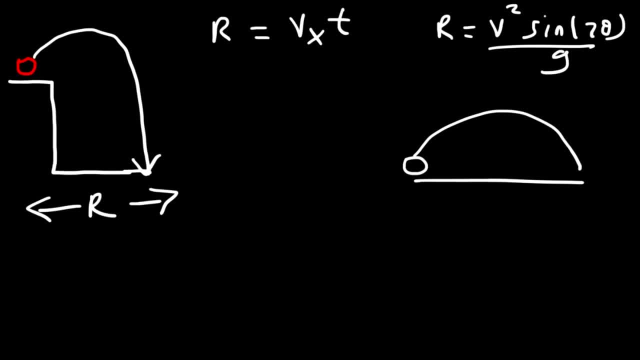 those two points and you don't want that. So to find the range for this type of trajectory, use the equation v x times t. Now keep in mind v x is equal to v cosine theta, So the range is simply v times. 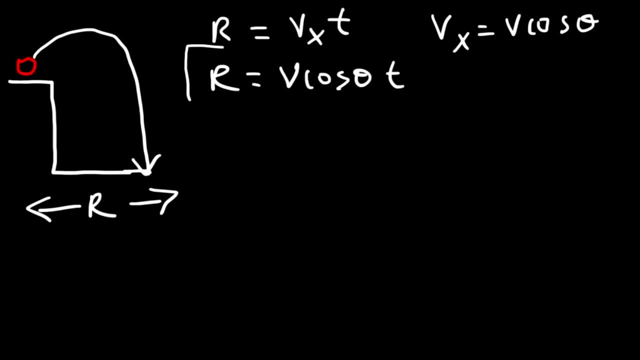 cosine theta times t. You can use this form of the equation if you want to, But you need to find the time it takes to go from A to C before you can use it, Which, using the last two equations, you can get that. 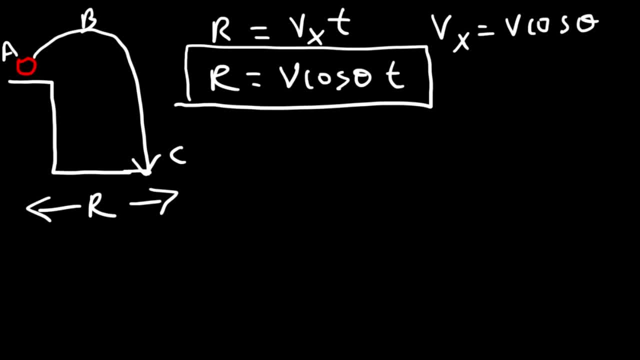 answer now And that's it. That's all you need to do to find the range Now. sometimes you might be asked to find the speed of the ball just before it hits the ground. So first you need to realize that v? x is constant. 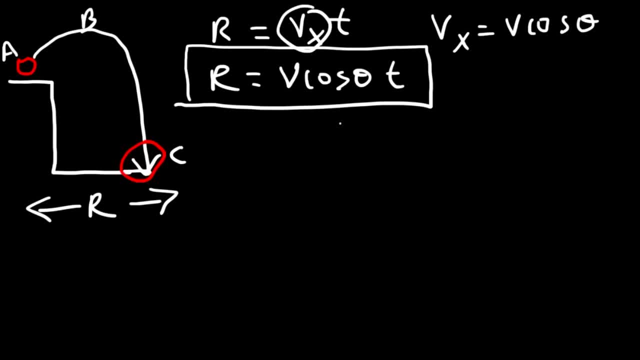 So whatever v x you have here is going to be the same at point C, At point A, point B and point C, v x is the same. So let me make sure I write that v x is constant. It does not change. So whatever. 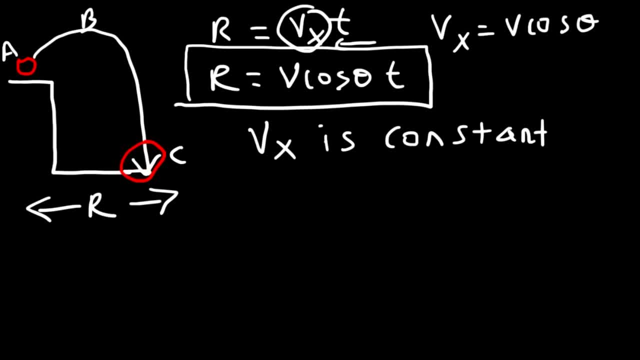 v, x you have here. we're going to use that to find the final speed of the ball just before it hits the ground. Now, just like last time we mentioned earlier in this video, we've got to find the vertical velocity as well using this equation. 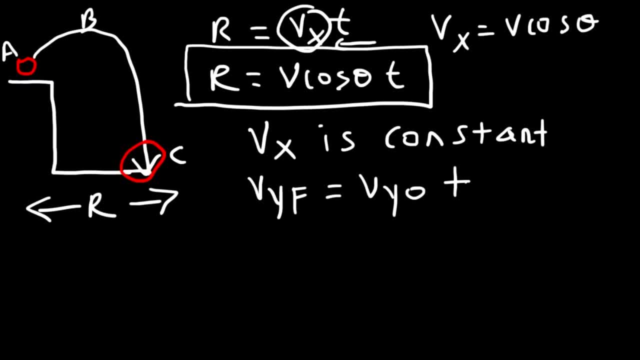 So you need to find v y final And you know v y initial is basically v sine theta, Where v is the initial velocity at point A And g. make sure you plug in negative 9.8.. T: this is the time it takes to go from A. 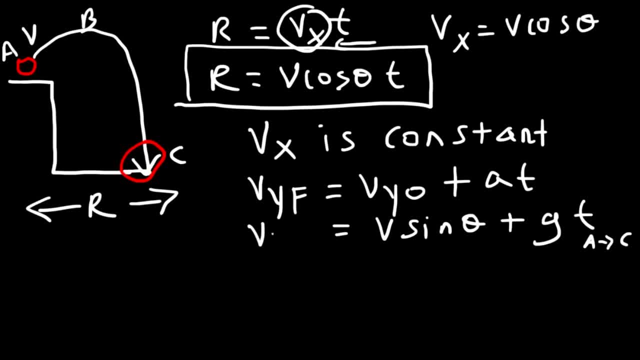 to position C. So use the total time. So this will give you the final vertical velocity. So once you have v x and v y at point C, to find the final speed just before it hits the ground, you can now use this equation. 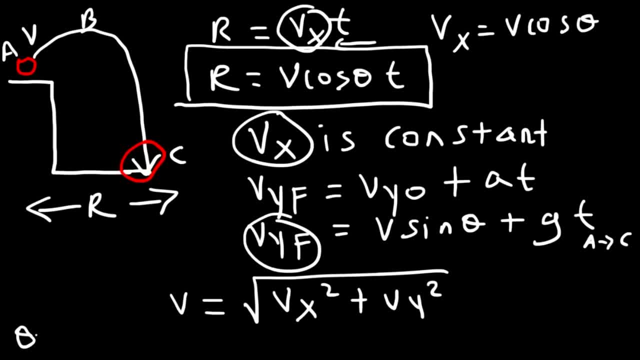 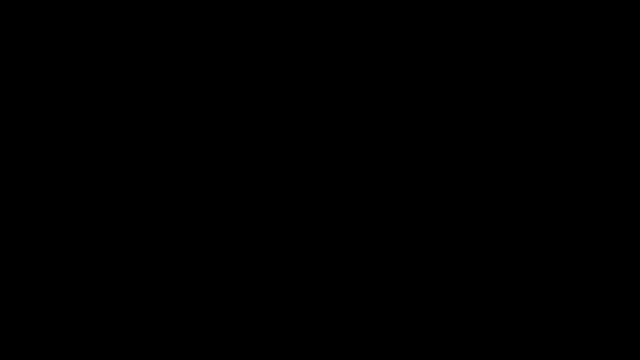 And if you need to find the angle, as mentioned before, it's going to be inverse tangent: v y divided by v x. Now let's talk about the angle. So let's say this is the ball and it's moving in this direction. 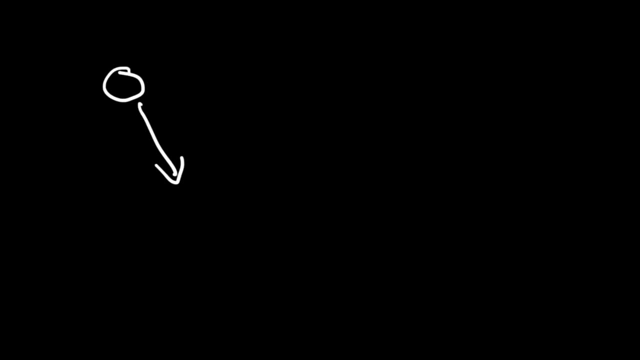 just before it hits the ground. So let's say this is the x axis and this is the y axis, Making the ball the center. So the ball has an x component, v- x, and it has a y component, v- y. You're looking for v, which is 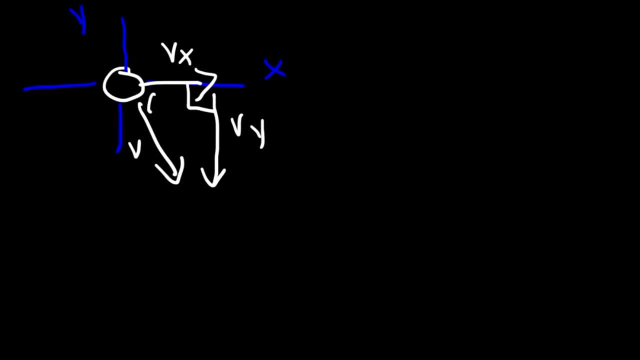 the velocity, and the magnitude of velocity is the speed. So once you use inverse tangent theta, make sure you plug in positive values for v y and v x, Even though v y is going to be negative. don't plug in a negative value, plug in a positive value. 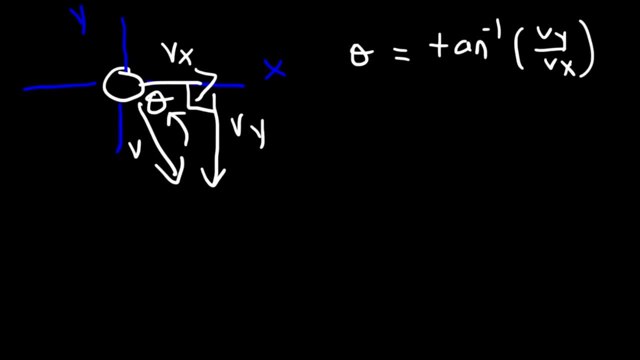 That will give you the reference angle, which is an angle between 0 and 90.. Now, sometimes you might describe your answer as being below the horizontal or relative to the positive x axis. So let's say, if the angle, let's say it's 60 degrees. 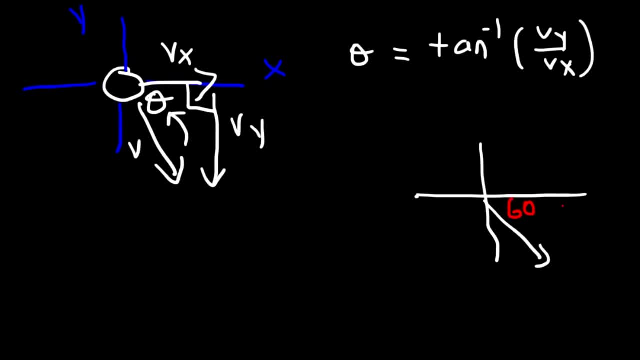 So that's going to be the reference angle. So you can describe it as being 60 degrees below the horizontal, which is the x axis, Or you could say it's positive 300 relative to the positive x axis. So you have two ways of describing the angle. 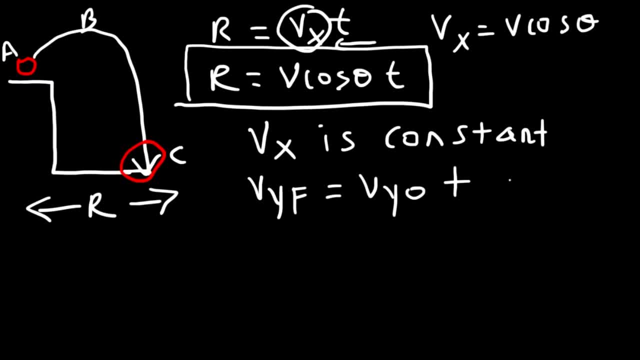 So you need to find v y final And you know v y initial is basically v sine theta, Where v is the initial velocity. at point a And g make sure you plug in negative nine, point eight T. this is the time it takes to go from a. 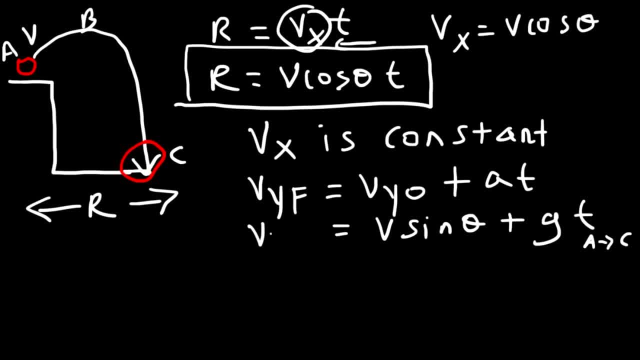 to position c. So use the total time. So this will give you the final vertical velocity. So once you have v x and v y at point c, to find the final speed just before it hits the ground, you can now use this equation. 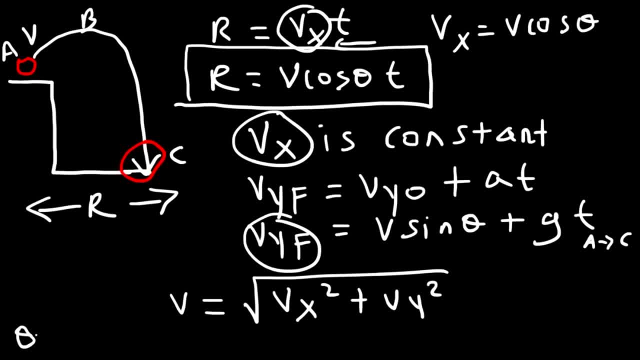 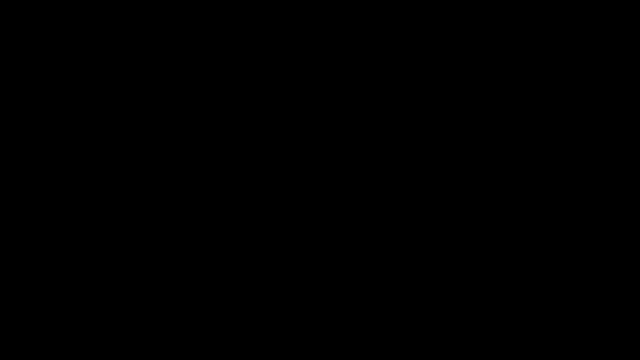 And if you need to find the angle, as mentioned before, it's going to be inverse tangent v y divided by v x. Now let's talk about the angle. So let's say this is the ball and it's moving in this direction just before it hits the ground. 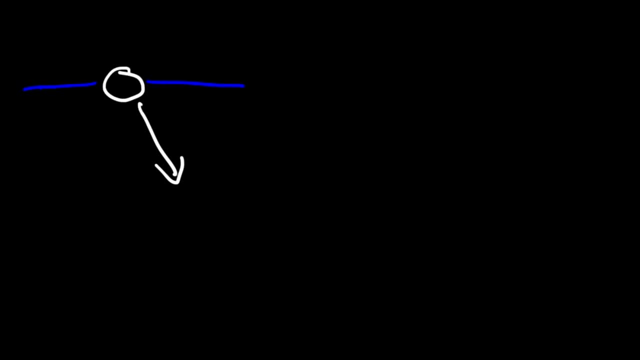 And let's say this is the x axis and this is the y axis, Making the ball the center. So the ball has an x component, v, x, and it has a y component, v, y. You're looking for v, which is the velocity and the. 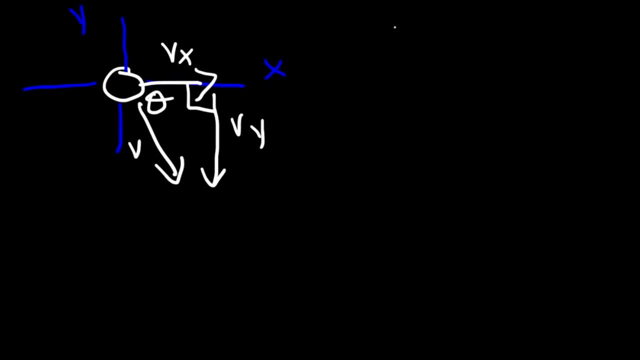 magnitude of velocity is the speed. So once you use inverse tangent theta, make sure you plug in positive values for v, y and v x, Even though v y is going to be negative. don't plug in a negative value. Plug in a positive value. 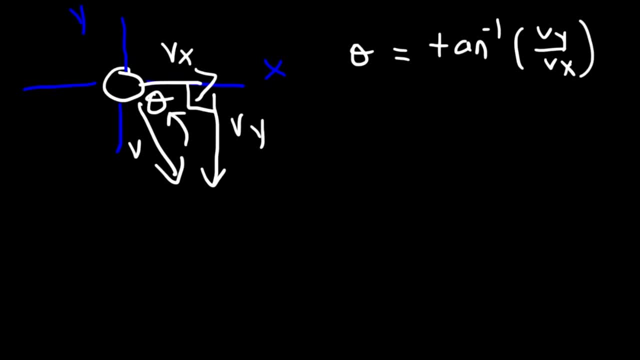 That will give you the reference angle, Which is an angle between 0 and 90.. Now, sometimes you might describe your answer as being below the horizontal or relative to the positive x axis. So let's say, if the angle, let's say it's 60 degrees. 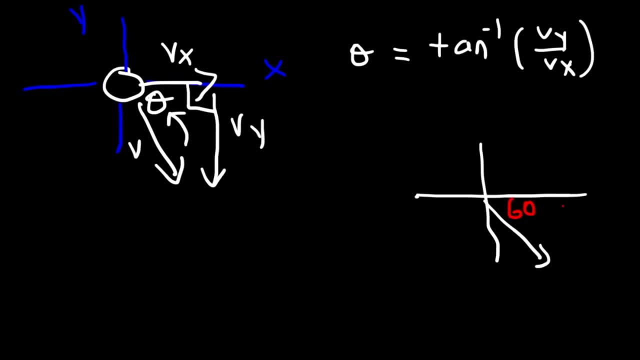 So that's going to be the reference angle. So you can describe it as being 60 degrees below the horizontal, which is the x axis, Or you could say it's positive 300 relative to the positive x axis. So you have two ways of describing the angle. 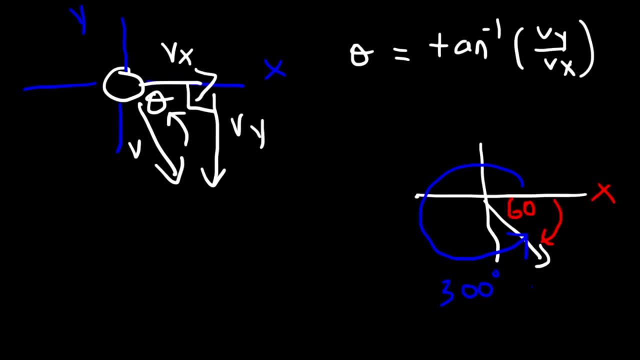 Just be careful to get it the right way in terms of the way the problem wants you to describe it. So it could be 60,, it could be 300.. Just think about what they're asking for If it's below the horizontal 60.. 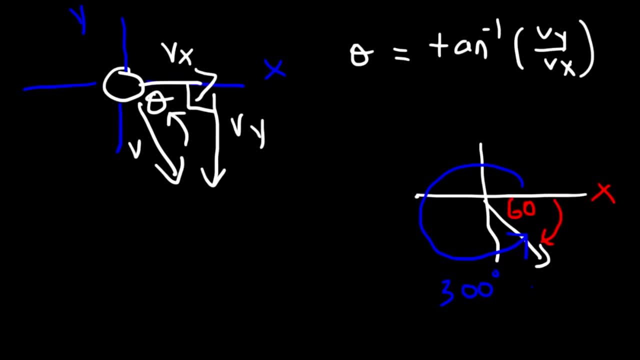 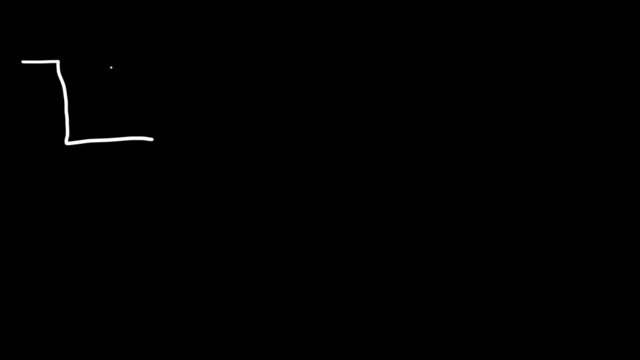 If it's measured from the positive x axis, then it's 300.. It's 360 minus 60, which is 300.. So make sure you understand all of the equations and when to use them. So just to review for this type of trajectory. 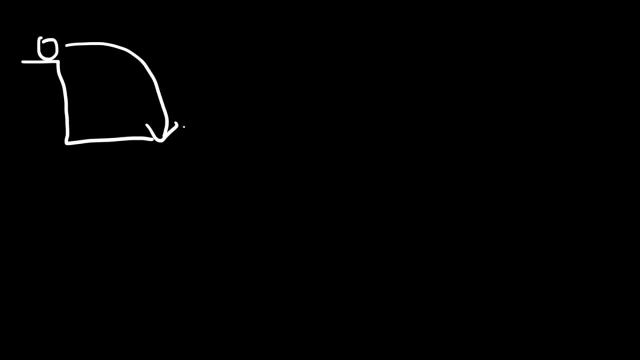 where the ball simply falls down. it travels horizontally from a cliff and just falls off. The height is equal to 1 half at squared And range is equal to vxt, And for all trajectories you can use this equation If you need to. 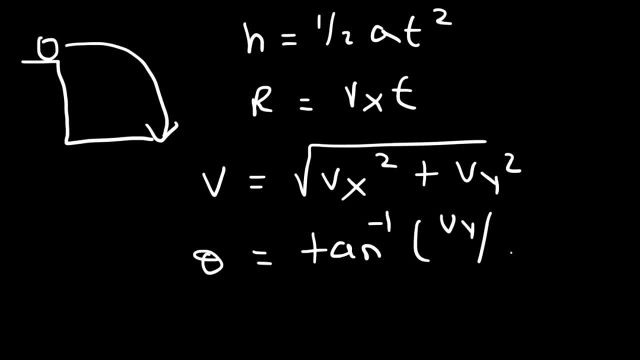 find the angle, use this: Just plug in positive values for vy and vx. And also, if you need to find vy final to use it here, use this equation. Now for the second trajectory. these are the main equations that you need. 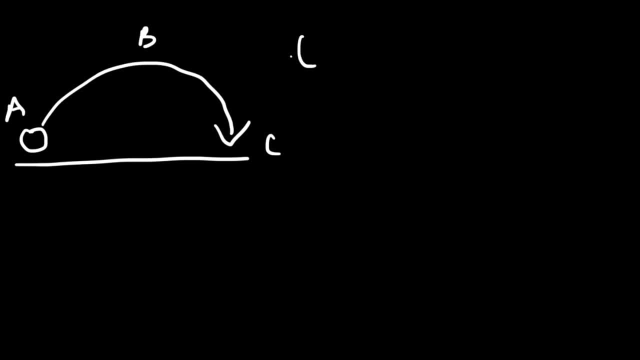 Just to review what we went over. So the time it takes going from, let's say, a to b- Remember it's just v sine theta divided by g- And the time it takes to go from a to c is twice that value. 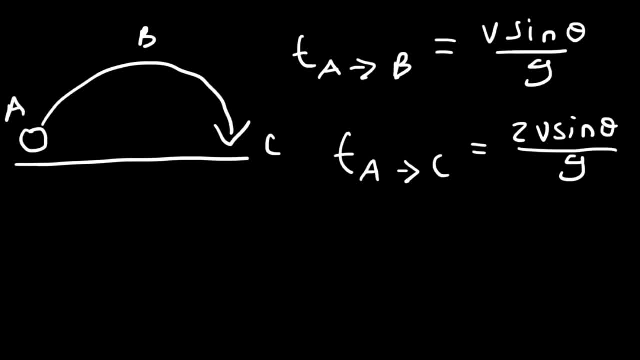 It's 2v sine theta Over g And the range is v squared sine squared divided by. let's see, if I remember this, it was no, that's not the range, that's the height. It was v sine 2 theta. 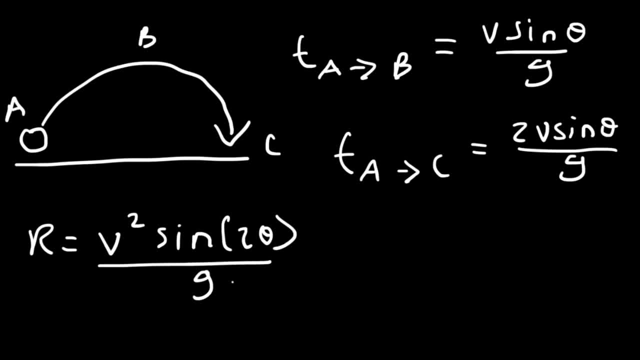 divided by g. That's what it was. And now for the other one, to find the maximum height. it's a v squared sine squared theta, divided by 2g. So those are the four main equations you need for this trajectory And also if you need to find the angle. 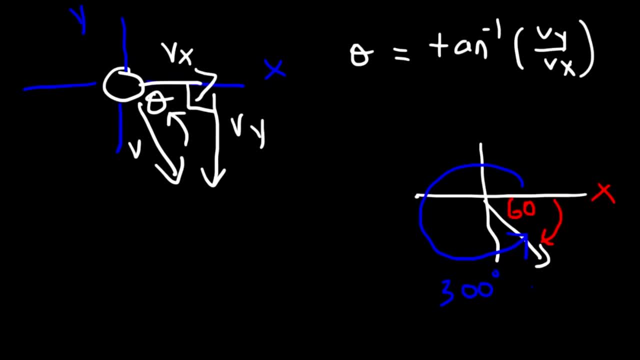 Just be careful To get it the right way in terms of the way the problem wants you to describe it. So it could be 60, it could be 300.. Just think about what they're asking for If it's below the horizontal 60.. 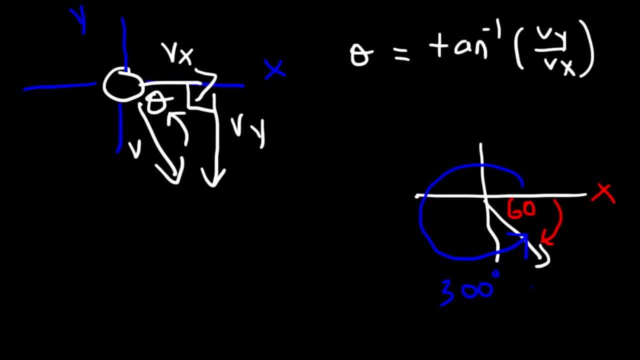 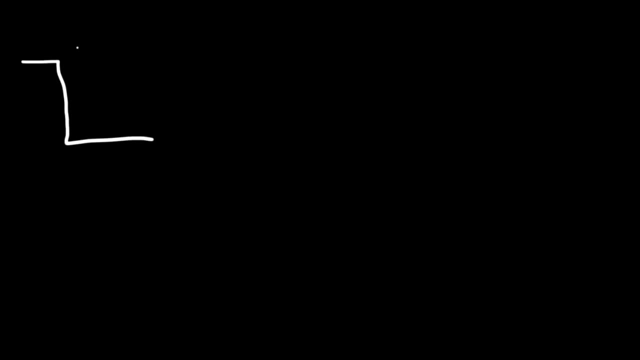 If it's measured from the positive x axis, then it's 300.. It's 360 minus 60, which is 300.. So make sure you understand all of the equations and when to use them. So just to review for this type of trajectory: 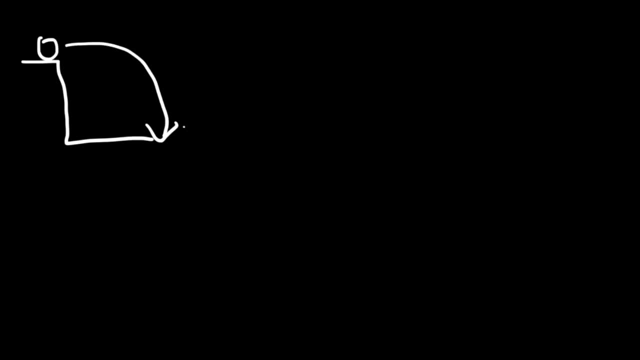 where the ball simply falls down. it travels horizontally from a cliff and just falls off. The height is equal to 1 half at squared And range is equal to vxt, And for all trajectories you can use this equation If you need to find the angle. 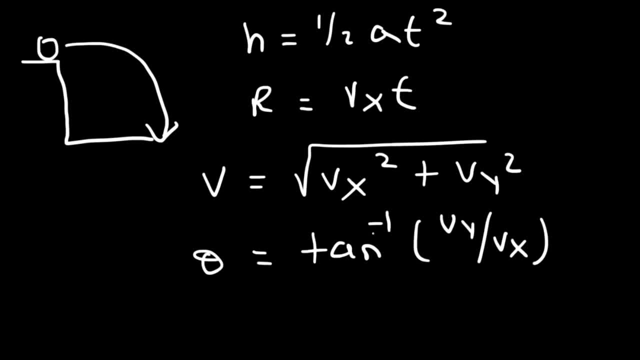 use this: Just plug in positive values for vy and vx And also, if you need to find vy final to use it here, use this equation. Now for the second trajectory. these are the main equations that you need, Just to review what we went over. 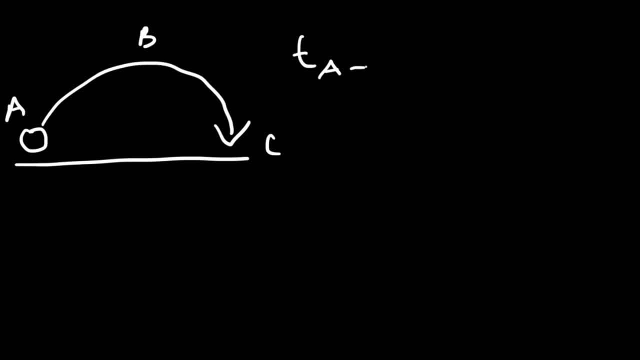 So the time it takes going from, let's say, a to b- remember it's just divided by g- And the time it takes to go from a to c is twice that value. It's 2v sine theta over g And the range is v squared. 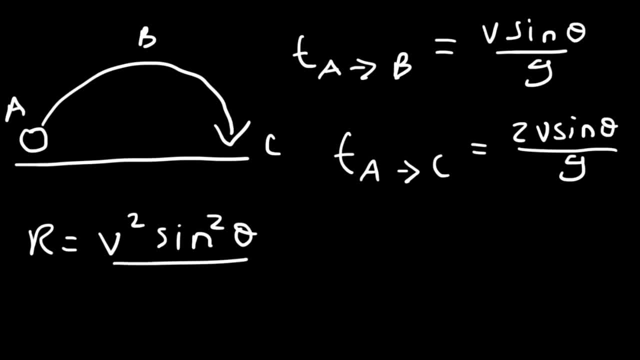 sine squared divided by. let's see, if I remember this, it was: no, that's not the range, that's the height. It was v sine 2 theta divided by g. That's what it was. And now for the other one, to find the maximum height. 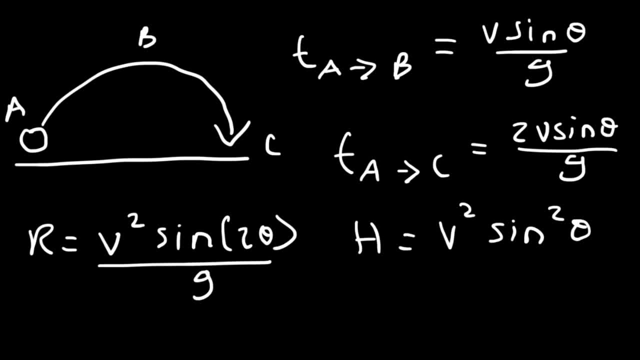 it's v squared sine squared theta divided by 2g. So those are the four main equations you need for this trajectory And also, if you need to find the angle just before it hits the ground at position c, it's the same as the angle.